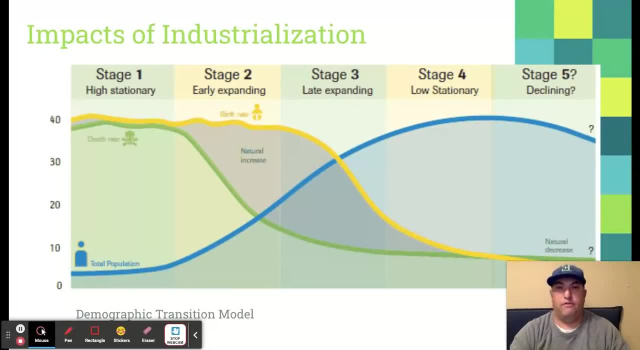 would make it to adulthood and they could have helpers to work on their farms. Because at this point many of the people who are living in the world are living in an agricultural, rural setting. industrialization changes all of that right. We start to see people moving away from those. 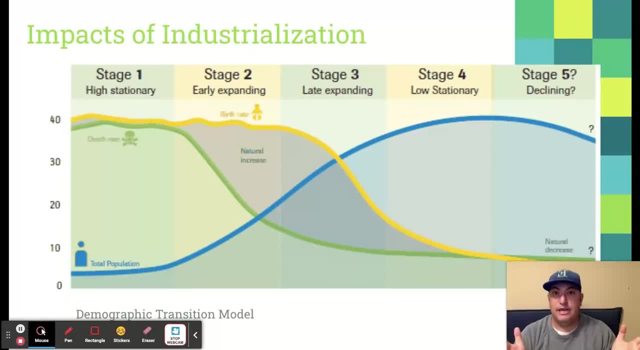 rural settings. They're not as necessary in those settings because of the agricultural revolution and they move to cities to find jobs in more industrial settings. all right, Because of that, and well actually before that, because of better sanitation, better healthcare, medicine. 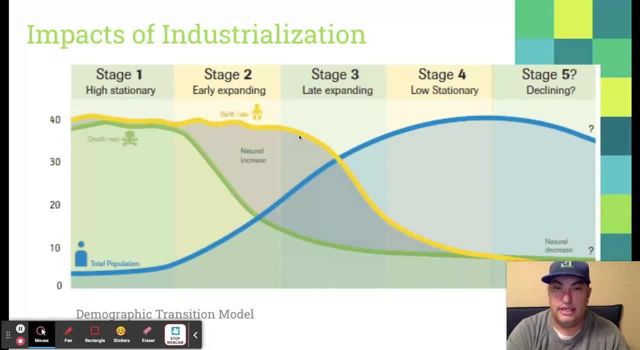 we start to see these death rates fall and then the birth rates also start to chase that down because we don't need as many people to work farms anymore. okay, But in stage two and stage three we see a very large increase of the world population. You see that with this blue line. 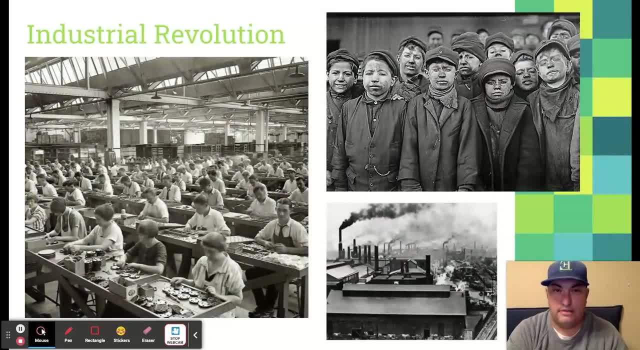 right over here. okay, So the industrial revolution, and I'll flash back to those photos right over here. this comes in around stage two and stage three of the demographic transition. all right, We're seeing a lot more people in our world. A lot of them are moving. 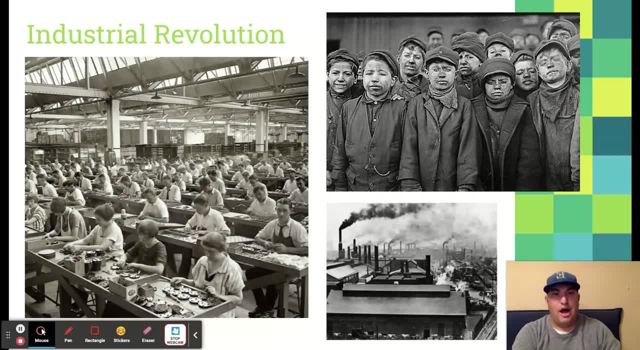 to cities and they're working in what are really like these dangerous factories: free jobs- and I'm not talking about like adults necessarily either right, This photo really spoke to me. You can kind of see how young these young gentlemen, these boys, are coming out of. 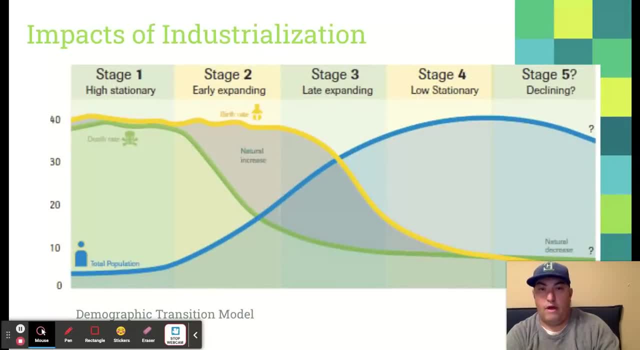 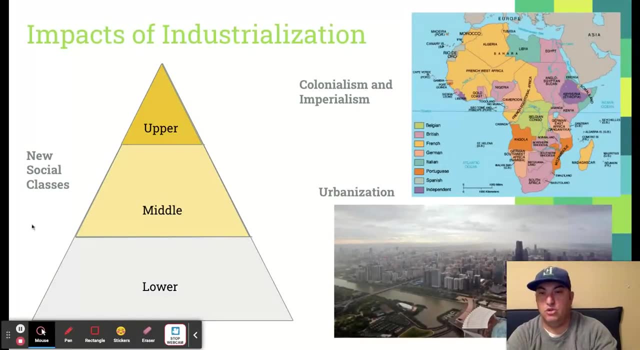 these factories in the 18th, 19th century. okay, All right, so let's talk more about some impacts of industrialization. okay, Over here on the left you can see a social pyramid. right, There was a middle class before the industrial revolution, but it wasn't as big or influential. 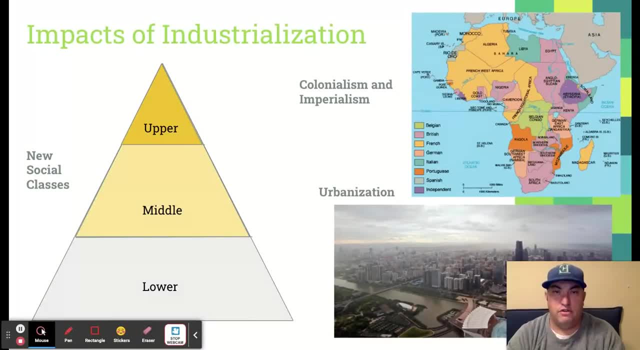 as the middle class that we see after the industrial revolution and especially the industrial revolution that we see in the world today. okay, Before we had like a nobility and basically a peasant class, but industrialization, that's a tongue twister industrialization really. 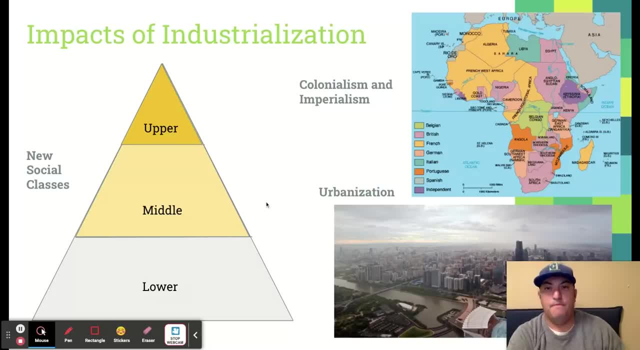 creates this strong middle class. okay, Now another impact: these investors who are putting in their money and trying to create more money. right, They need markets, They need resources, They need raw materials. so colonialism and imperialism was also going on. 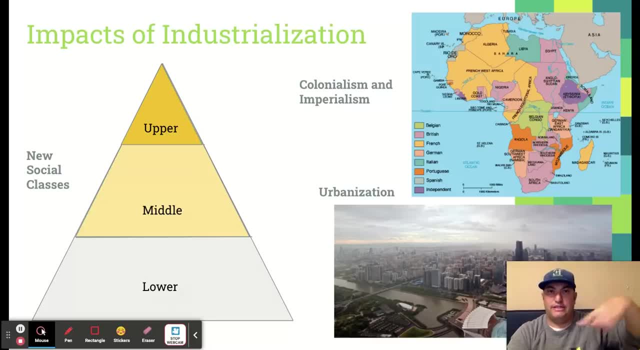 before the industrial revolution, but this kind of like accelerates it a little bit. right, These mainly European countries need a lot of things to make their things so they can sell their things, and other places have those things so it makes sense for them to go take over places in Africa. 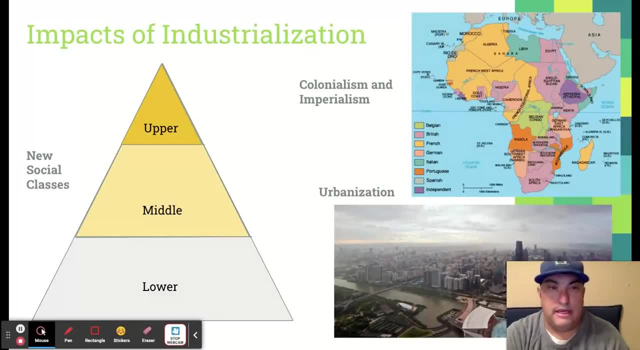 or Latin America, or in parts of Southeast and Eastern Asia, okay, And the Middle East as well, and then you also see urbanization as well, as we've mentioned. so a lot of these again flashbacks to previous units. That's one of the things I love about this. 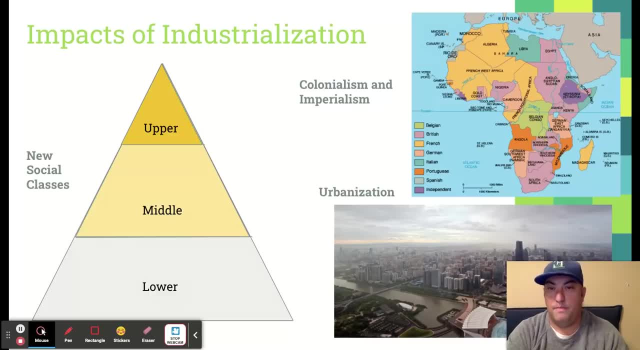 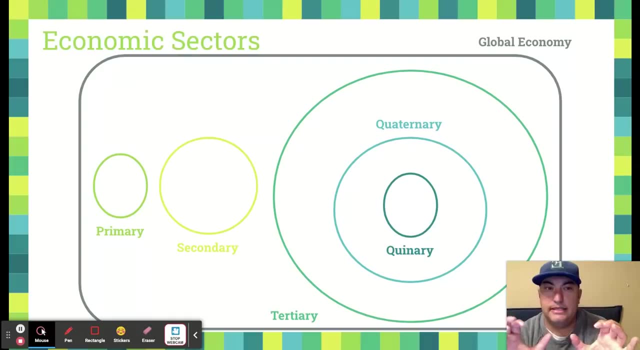 unit is that there's a lot of callbacks to stuff that you should already know. All right, let's talk about economic sectors. This is some new stuff, right? The global economy, the way you should look at this graphic organizer that I made, this image that I made. 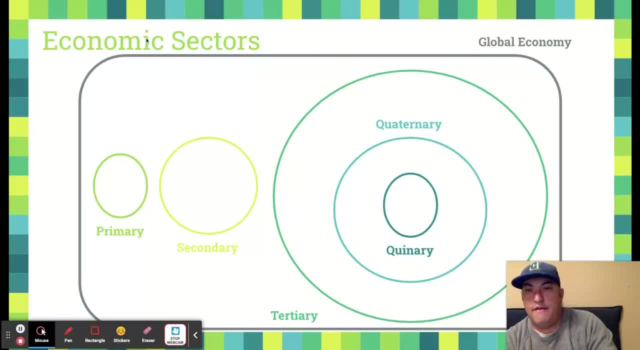 is kind of like a Venn diagram. okay, So everything was within the global economy. That's like this rectangle right over here. okay, We start off with the primary sector. Primary sector work has to do with extracting and collecting raw materials, right, So think farming If you're in like a coal. 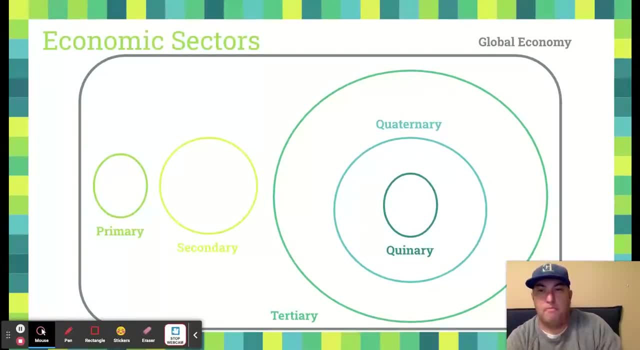 mining industry. those are going to be primary jobs, jobs in the primary sector. okay, Now, once we take these raw materials and we start doing stuff with them, we start processing them, we start turning them into actual raw material that's going to go into something else, that is, the secondary sector. 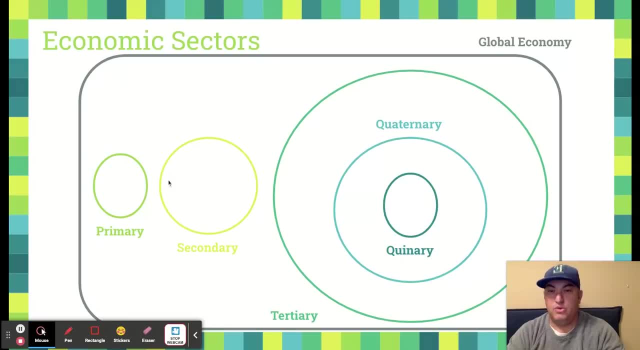 right over here. okay, So you see there's no real overlap between the primary and the secondary sector. okay, Now this big circle over here in the green. this is the tertiary sector and this is all about services. okay, Service jobs are what the majority of the American economy 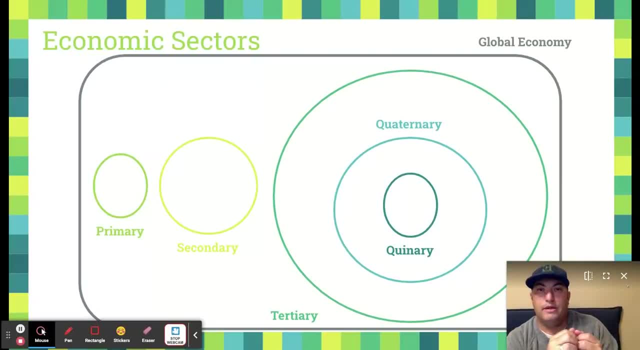 today is made out of right. People mainly go to work doing something for somebody else, right? We don't have that in the United States. Our secondary sectors are decreasing very rapidly and that's because most people are working here in the tertiary sector doing some sort of service-oriented 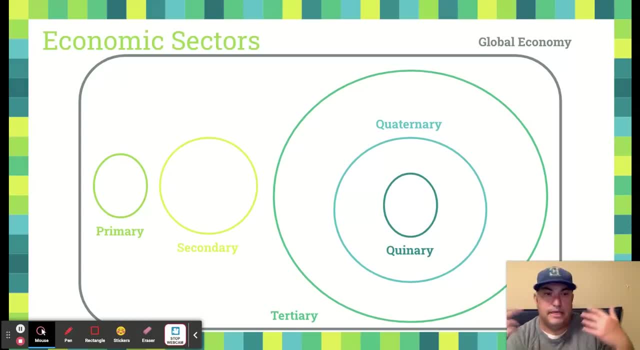 job right, And that could be lots and lots of different things, from teaching real estate, working at a restaurant, if you're a lawyer, if you work in healthcare- all of those are services okay. Now, within the tertiary sector, there's two more sectors. okay, You have this light blue. 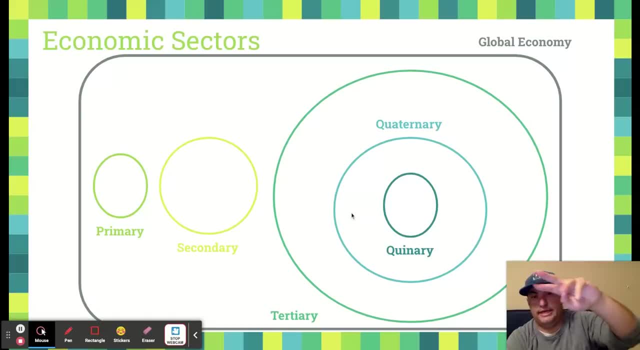 circle, and that's called the tertiary sector and that's called the tertiary sector and that's called the quaternary sector, quaternary or fourth sector. right Now, this has to do with the sharing, processing, researching, cultivating of information. okay, It's a little bit vague. 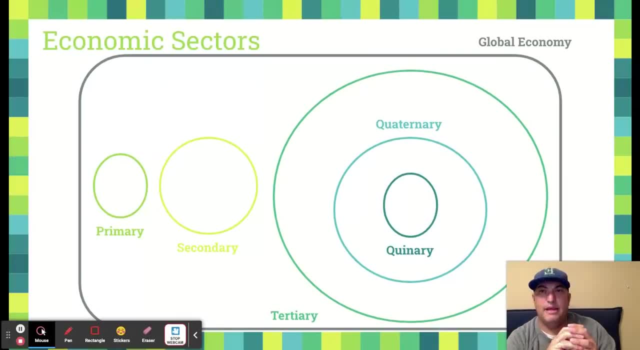 but I haven't really found the best definitions for these last two sectors. but essentially anyone who deals with like the creation or the maintenance of information is going to be in the quaternary sector, and then within the quaternary sector you have the quinary. 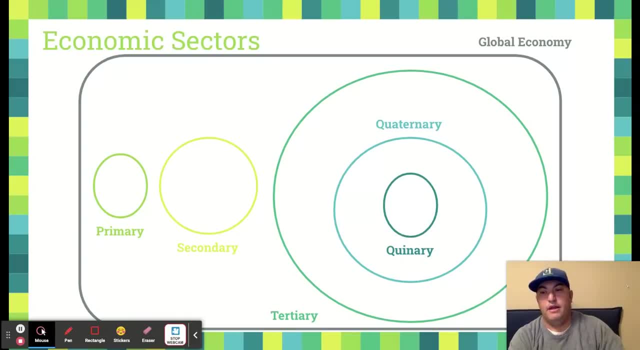 or the fifth sector, and these are your big decision makers, right? The quinary sector is all about the people who take the information that's produced and collected in the quaternary sector, and they have to decide what to do with it, right? So these are going to be your CEOs. 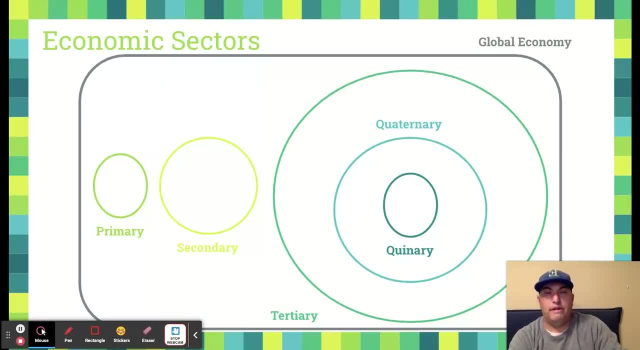 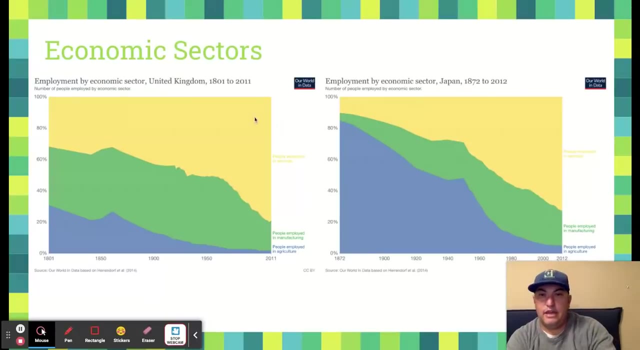 politicians, people like that who are relatively powerful, are going to be working in the quinary sector. okay, Now, before we move on, or actually as we move on, well, I'll show you this one, this yellow on this graph: this is the tertiary sector. green is going to be the secondary sector. 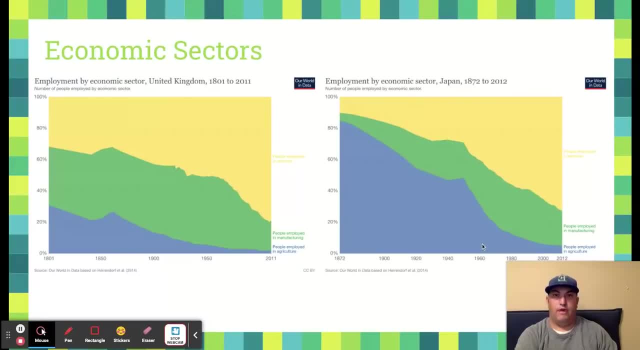 and blue is going to be the primary sector, right? There's a lot more money to be made in the tertiary sector, okay, So we have two different countries here. on these two graphs from shout out to one of my favorite websites for teaching AP Human Geography: 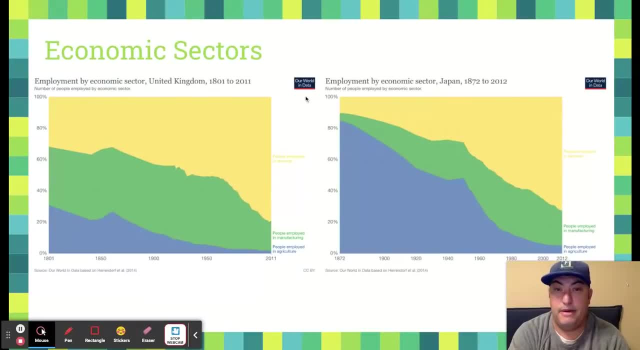 Our World in Data, or just Geography in General, right, Our World in Data. if you haven't been to that website, awesome, awesome, awesome visualization And graphs that are going to help you understand the content here, So I chose out these two. 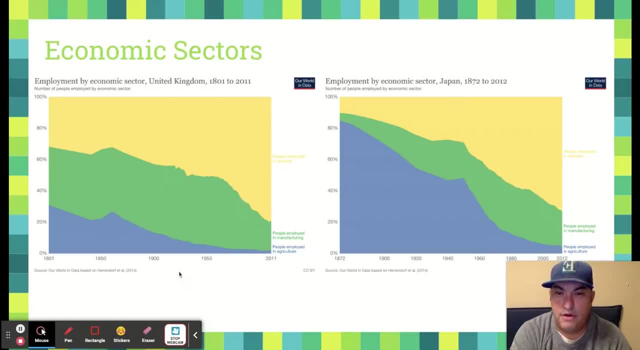 for both the United Kingdom and Japan. Now you'll have to notice here that the x-axes right. I'm not a math teacher, don't make me teach you math, but the x-axes on both of these graphs are different. right Over here in the United Kingdom we're starting way over in 1801.. 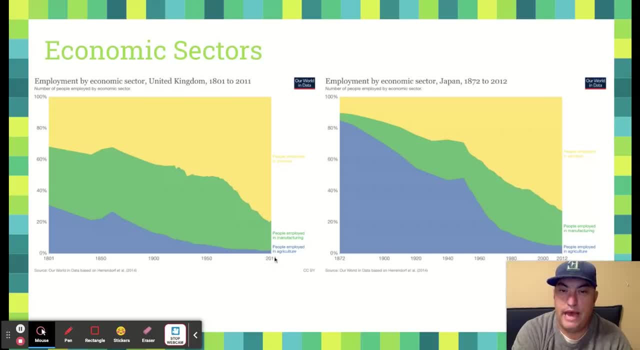 In Japan, we don't start until 1872, right, We end in almost the same place though: 2012 for the Japan graph, 2011 for the United Kingdom. Okay, Now, hopefully, your teacher told you that the Industrial Revolution started in the United. 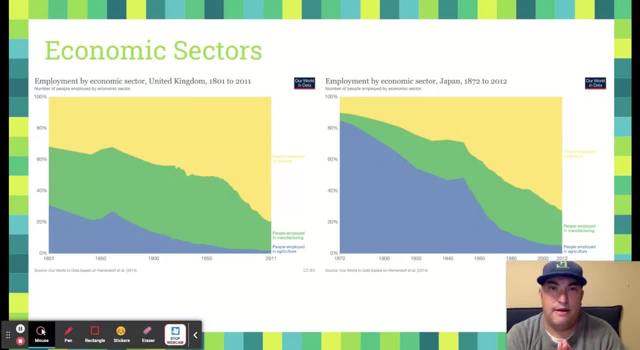 Kingdom started in Great Britain. right, Lots and lots of reasons for that. I'm not going to get into all of them now, but mainly water, water. It always comes back down to water with the Industrial Revolution. Do some research on that. It might come up on the test. okay, Anyway, the United. 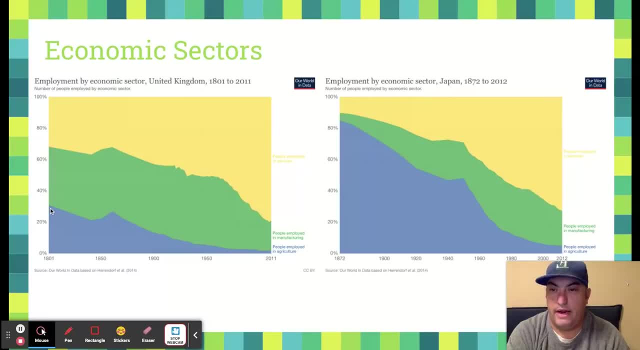 Kingdom, the very first country to industrialize, right. So you can see that their blue sector right here, the agricultural sector, the primary industrial sector, the primary industrial sector, it's a very small percentage of their employment, even way back in 1801.. Maybe, like what? 30% right. 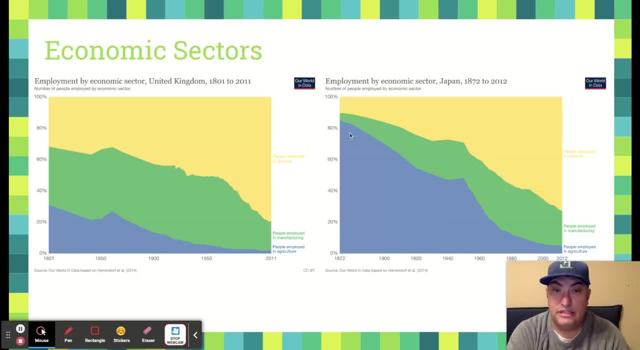 there In Japan, when we start here in this graph in 1872, it's over 80%. okay, But you can see, for both of these countries this primary sector falls fairly rapidly through the ensuing decades and centuries, right The manufacturing sector, that secondary sector, it becomes very big and then 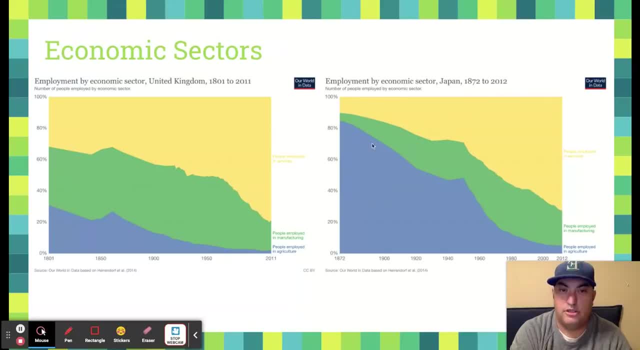 starts to slow a little bit, And you're starting to see more of that slowing in the modern world today. And then your tertiary sector just takes off in both of these places. all right, Like I mentioned before, there's money to be made in this. 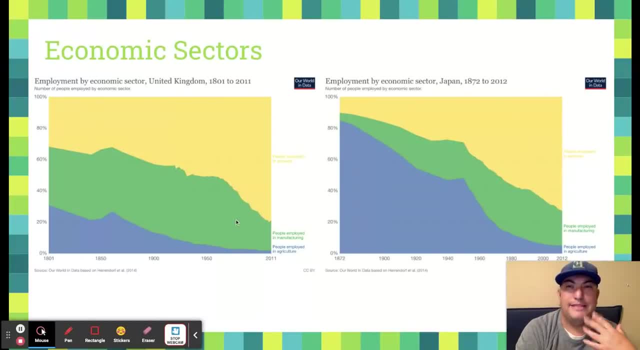 tertiary sector. But this is kind of like- almost like a sector transition is how I would kind of call it. So that's not like an academic word, That's something I'm inventing. But you're starting to see these countries go through this industrial sector transition as well, where they're moving away from the primary 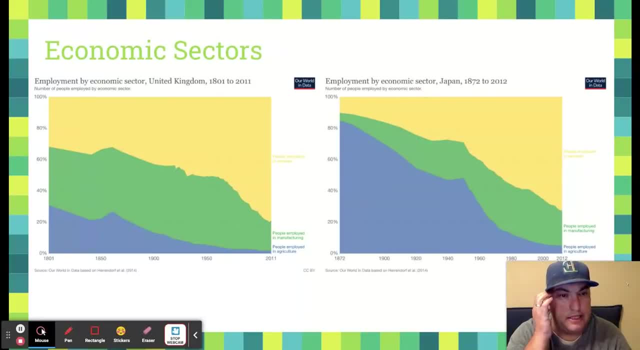 sector Towards the tertiary sector, And I think these two graphs show that very well. okay Now, obviously the United Kingdom did it first. They're the first country to industrialize. Japan didn't really get into it until the 20th century. Some countries aren't even there yet, right? Unfortunately, our world in data only has like a dozen. 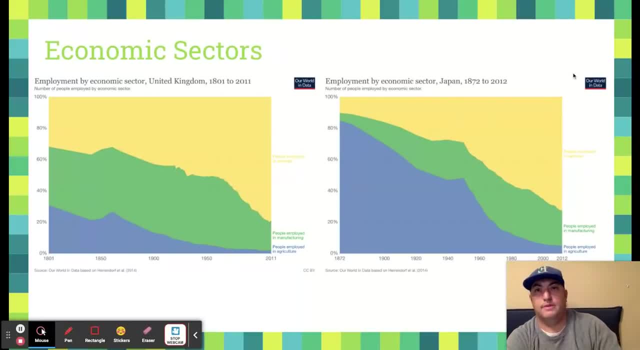 countries for this graph. But if you were to look at some of your sub-Saharan African countries, some of the smaller countries, some Eastern countries like East Asian countries, they're not quite here yet. Hopefully they'll get here in the next few decades. But this doesn't apply to everybody, because not every country is done with this. 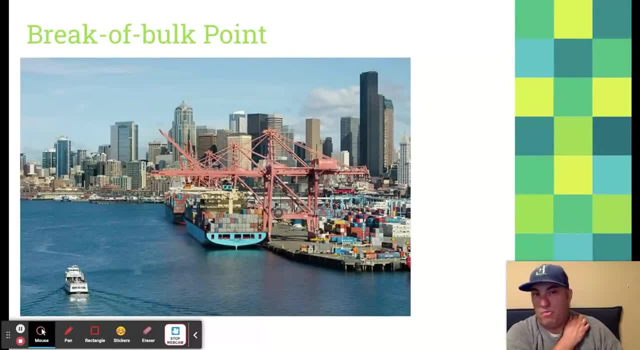 transition yet. okay, All right, Let's talk about Break of Bulk Point. A lot of this unit has to do with our stuff and where our stuff is coming from, And one of the places in the economic landscape that makes that possible is this Break of Bulk Point. okay, So this is the port of. Seattle, Seattle, amazing city, Probably my second favorite American city out from San Diego, the North Pole, but then in a minute it'll be built into Seattle. So and now let me just talk a little bit about, And this is our session, where we're BEC- hopefully I hi. mm-hmm. I mean this is important. So when I first put it, the jungle, this group, you don't like it, But this partnership, we just put it together Right now, this whole Lookport, build up this W? I. 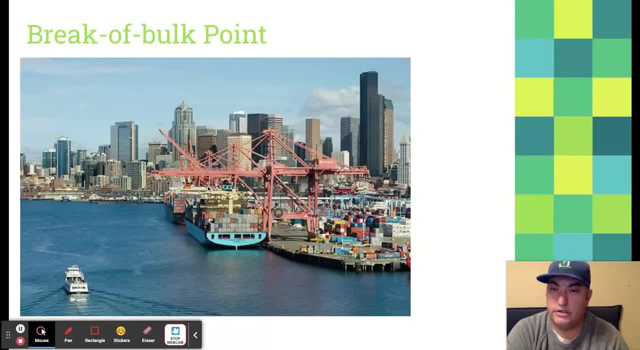 out after San Diego and they've got one of the busier ports on in all of the Western United States and you can see the port here. you see these containers right when you order stuff on Amazon, usually like gets shipped across the world somehow on one of these container ships and then it gets unloaded by the. 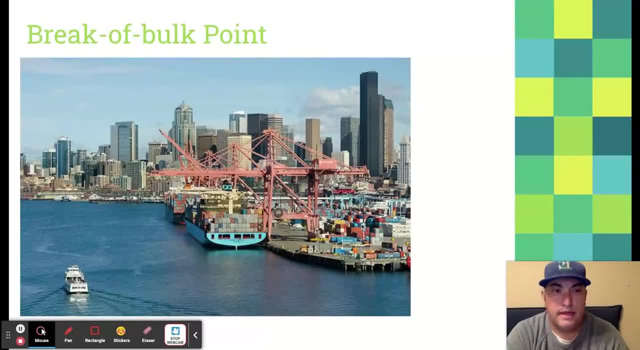 cranes and then breaking down, broken down right like something that somebody's gonna go in here and open up the container and break down all the bulk, right. that's what a break a book point is okay. all right, let's talk about least cost theory, these cost theory here. this is Alfred Weber. I don't know why he. 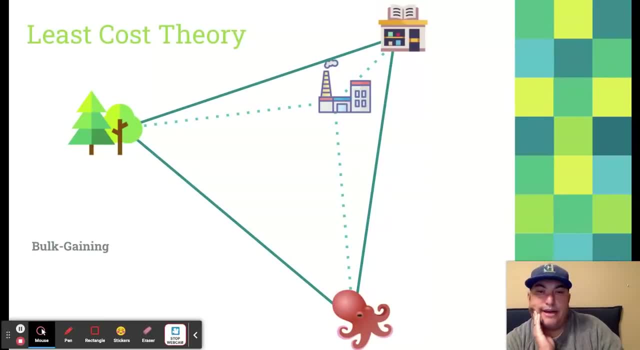 didn't get the shout out in the in the course in the exam description, but but he's our guy here for these cost theory. okay, now I'm just disclaimer. before I get into this I'm gonna oversimplify a lot here. okay, a lot, I'd be ready be. 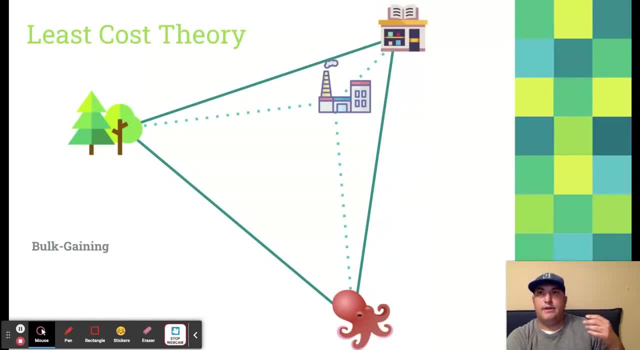 ready, but we're oversimplifying. okay, now, least cost theory is all about deciding where your factory's gonna be. okay, that's what this icon is. it's a little factory and in this situation, we're gonna assume that I am going to be making books. okay, I'm making books, and 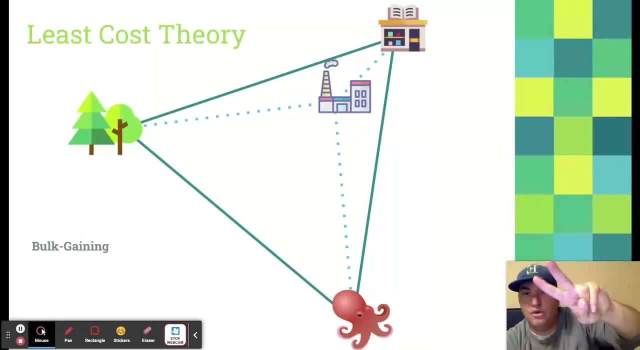 we're gonna again oversimplify and say that there's only two things that need to go: in the book, right, the paper which we get from wood, from a forest, and in the ink so we could print the words with right, and we're just gonna assume for a 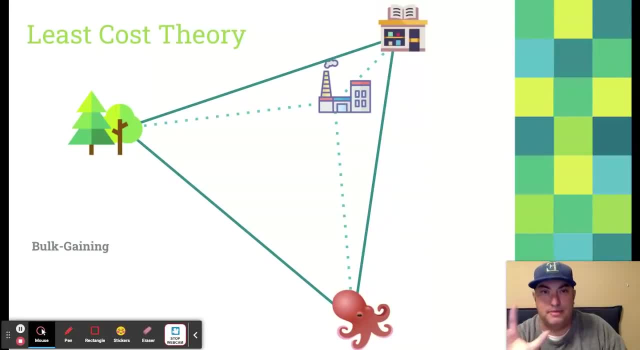 second, again oversimplifying, we're gonna assume that I get my ink from octopuses. right, don't go reach for your nearest book and assume that there's octopus ink in there. there's probably not. I'd be surprised if there was, but let's just go with this analogy right here, okay. 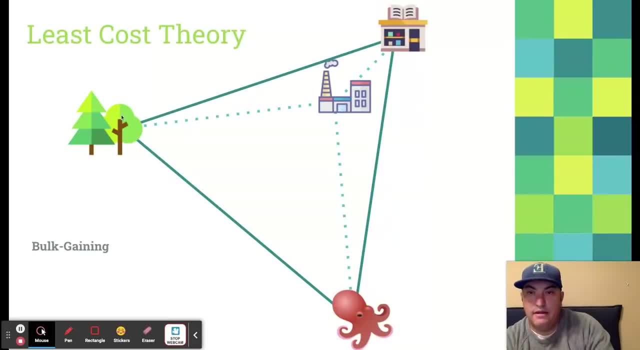 now the factory is gonna be where I take the wood, turn it into paper and I take the octopus ink and I get it onto the pages and I have my book right now. this is what is gonna be. this situation is gonna be called bulk of gaining. okay, 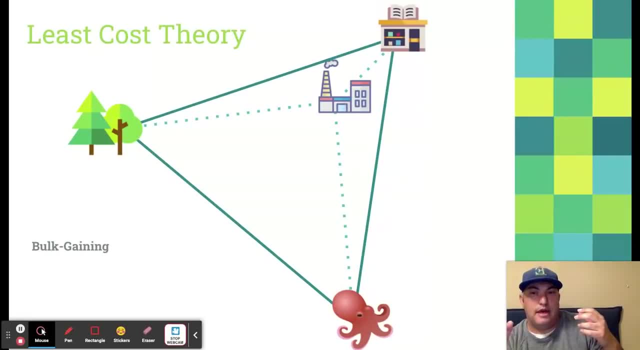 because, believe it or not, in this situation like the, the, let's assume that I'm getting the paper already. right. this, this, this resource, is coming to me as paper already. I don't need to cut on the paper, but we're adding ink to the paper, right? so this thing is getting bulkier, right, the materials that are on being. 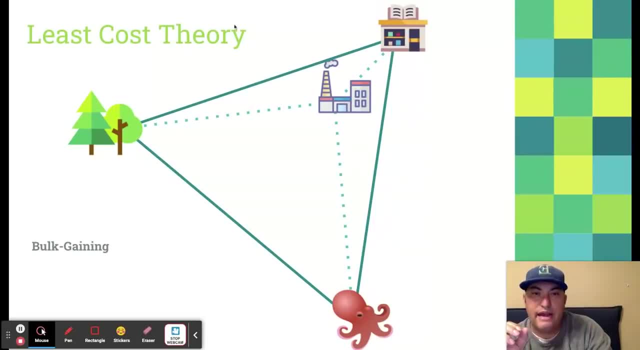 put together to create my final product are both lighter than the actual final material itself. so this is called bulk gaining right now, since the heaviest object in this whole creation right is the book. since it's heavy, I don't want to have to pay to transport it very far, so I'm gonna put my factory way up here. 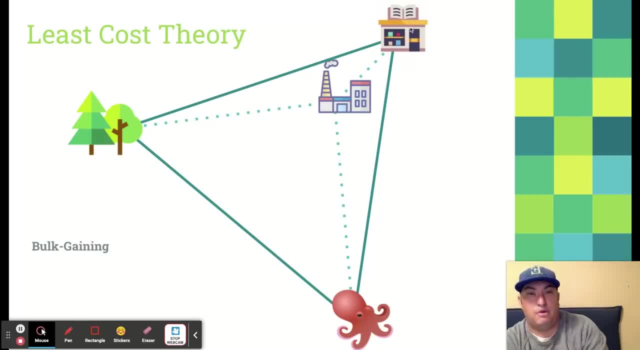 close to that market, right close to where I'm gonna sell this product, in this case, where what I'm selling to is obviously a bookstore. okay, um, now, this is different from a bulk reducing industry. okay, now, let's, in this example, say that I am creating furniture, I'm creating furniture, I'm creating furniture. 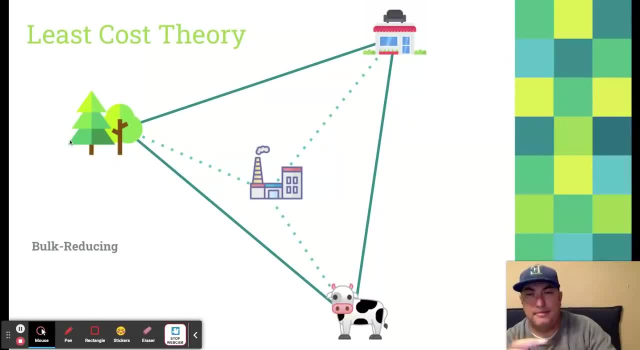 okay, so I need the wood on. it's gonna be like the frame of my couch or my chair, whatever. and then I have the leather. right, that's what this cow represents. I'm getting getting some leather from this cow right now. those raw materials are actually gonna be heavier, right? I'm getting the big. 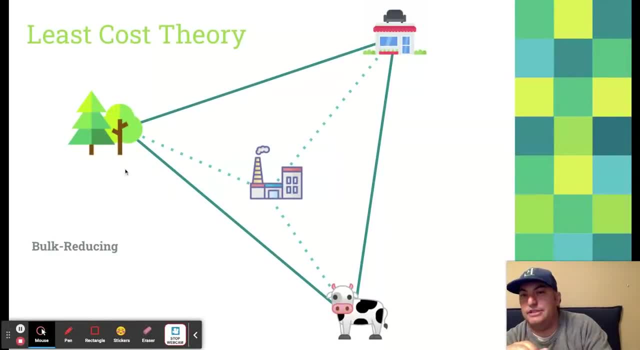 leather hides from the cow and getting lots and lots of trees to break down into the frames for the for this furniture. so this is gonna be a bulk reducing industry and according to Weber, on favor, its favor. I don't know Weber w-e-b-e-r, but since it's bulk reducing, 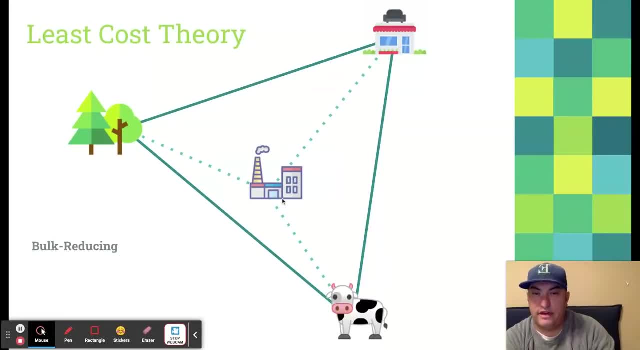 um, I'm gonna put my factory here closer to my raw materials, so this actually becomes the shorter trip, right, because this is the heavier stuff. I'm not gonna mind making this trip and transporting my furniture all the way up to the furniture store up here, because it's gonna be lighter than the raw materials. 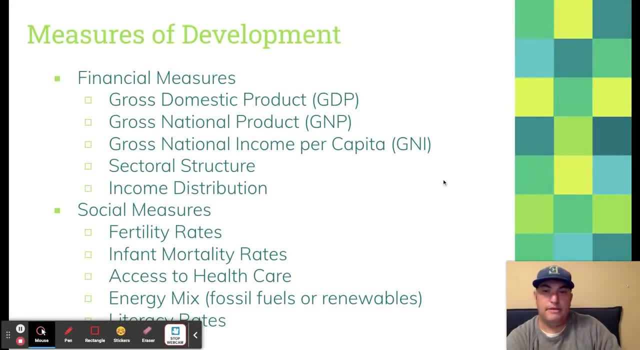 okay, that's least cost theory. all right, measures, the development. sorry guys, sorry, there's no cool fancy image, no icons here. this is just words, right, but when we are talking about different countries around the world and how developed they are, there's lots of things, lots of statistics really, that geographers take into account. okay, five. 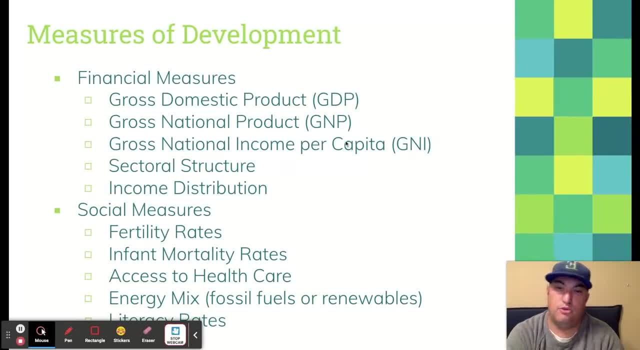 of these are financial measures: gross domestic product, gross national product, G&I sectoral structure, which we talked about, and in the distribution of the income of the people who are selling their products and have no income. the people who are selling their products and have no income. 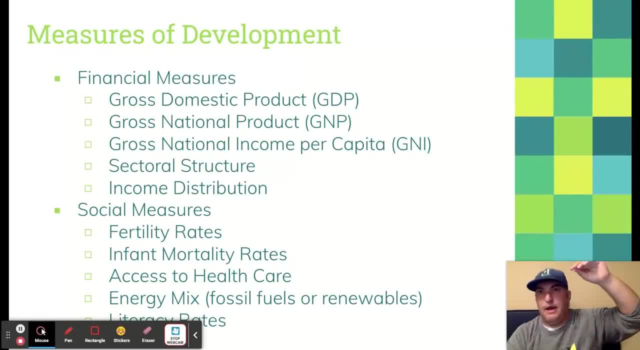 within the country right? Is the top 1% making- I don't know- 20% of the income? Is the top 1% making 50%, 70%, 80%? Does that sound like a lot? It is a lot right, But that's what we mean with. 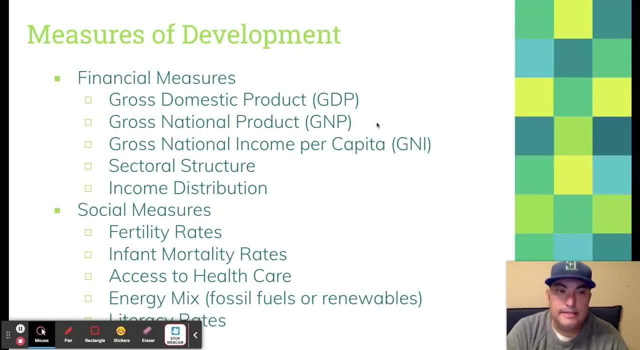 income distribution. okay, I'm not going to get into all of these because that's probably like another 45-minute video, But just know that these are the statistics that geographers use And essentially it's like how productive economies are. okay, That's it. I'm not going. 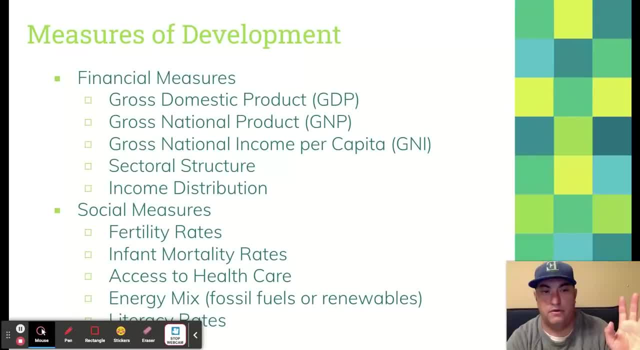 to go into them. I'm not going to go into them. Go find Jacob Clifford right, He's the econ guy. He'll tell you all about those ones. okay, Now, beyond financial measures, we also have some social measures. Some of these should also look familiar to you from back in Unit 2. Fertility. 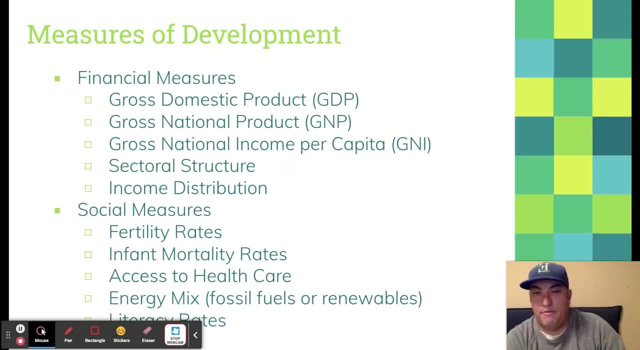 rates. how many people are being born per woman? infant mortality rates. how many of those kids are able to make it to their childhood access to health care? how many of those kids are able to make it to their childhood access to health care? how many of those kids are able to make it to their 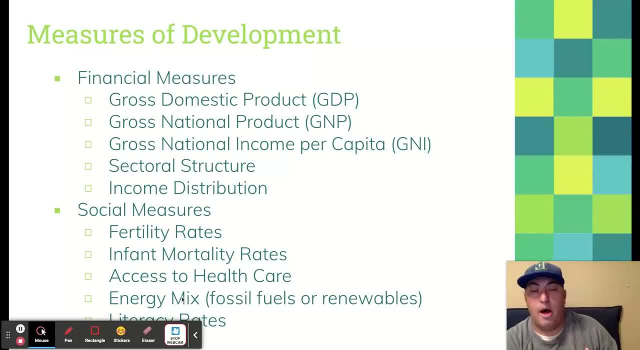 childhood access to health care. energy mix: There's some really cool graphs on Our World and Data about energy mix- right, My class took a look at some of those. So our country is using fossil fuels or renewables- okay, So go check those out if you get a chance. And then literacy: 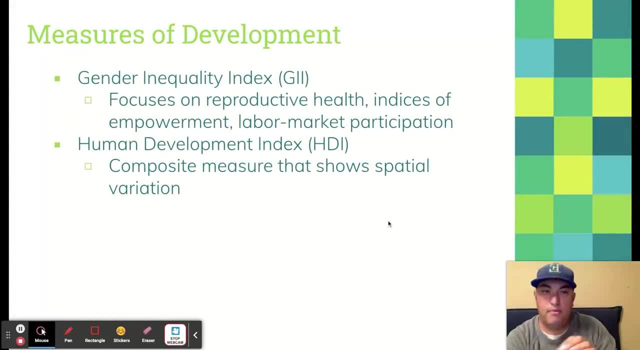 rates is our last social measure. okay, A couple more that geographers focus on. There is gender inequality index- It is what it sounds like, right, How equal are women to men in that particular country? And then human development index is kind of like our composite right It. 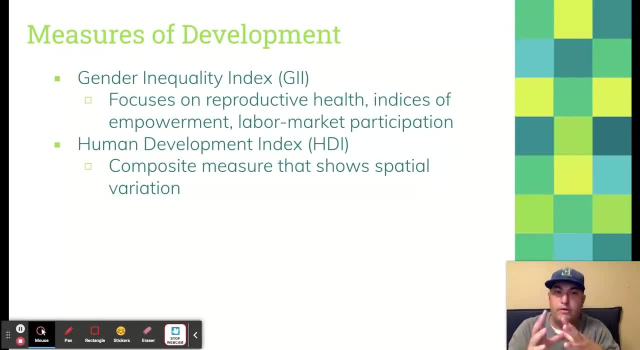 takes a lot of these other measures and puts them all into like a single number And I believe the closer you are to one is where you want to be right. The closer to one means you're more developed. The closer to zero, the less developed you are okay. So essentially what I think the most: 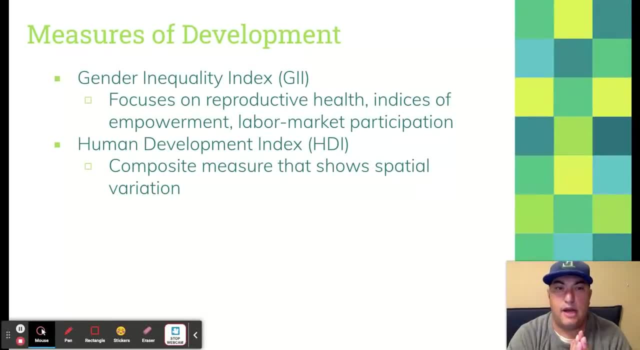 important thing for you to know is that these are the statistics that geographers use when they want to really measure how developed they are. So I'm going to go ahead and show you a little bit of what the country is. Is it very far along in the demographic transition? Is it making a lot of? 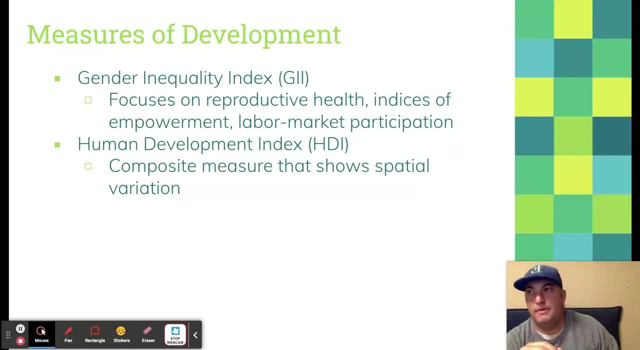 money like a United States or like a Japan or like a Germany, Or is it kind of like on the way there, like a Mexico or an India, Or is it like kind of very far behind, like I don't know, maybe like Ethiopia, Somalia, Cambodia, Just kind of guessing on those ones, Sorry. All right, Women and 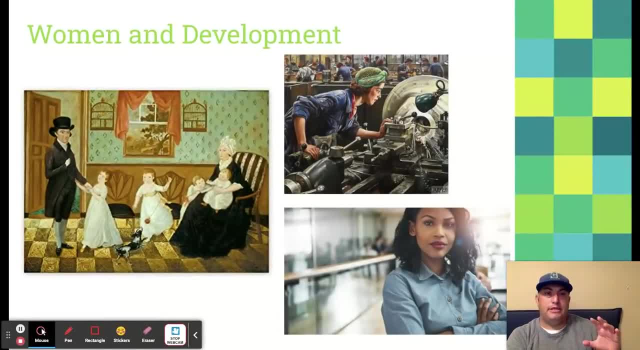 development. okay, Now, this is kind of a couple of things that I want to talk about. I want to talk back to unit three right here, But what you should be, I think you should know for women in development is that gender roles and the expectations that we have of women plays a very large role in how 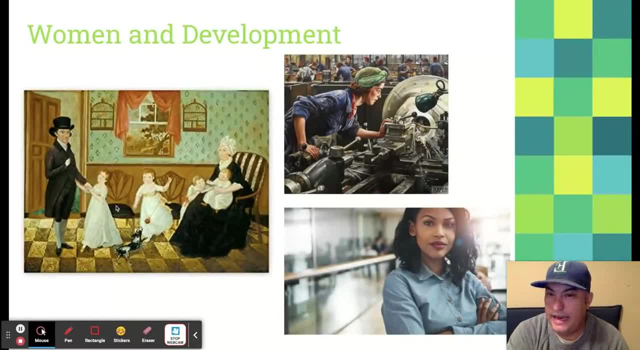 developed a country is right. If women are expected to be caretakers and mothers and that's about it, that's not going to be very good for a country's development. right. If they're able to move into a more industrial job or, even better, like a tertiary sector job, then in the long run 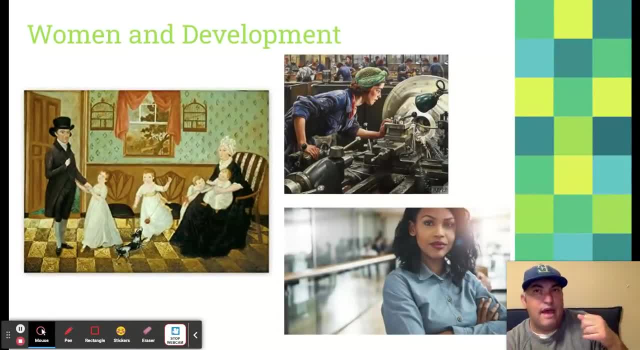 that's going to be better for a country, because, because the way I see it, it's going to be better for a country's development, right, And I think that is that every person is kind of like a little economic engine, right, And if you're relegating women to just being a mom and a caretaker, not, 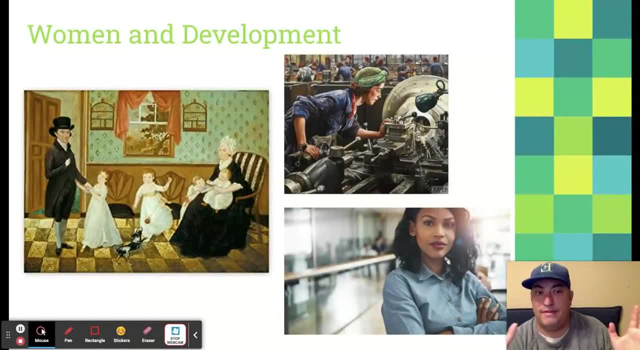 not that there's anything wrong with that right. I love my mom, I love my wife. They do a great job of being a mom and a caretaker, But there's so much more potential there that that our previous societies never tapped into, And I'm glad to see that in our modern world, our gender roles are. 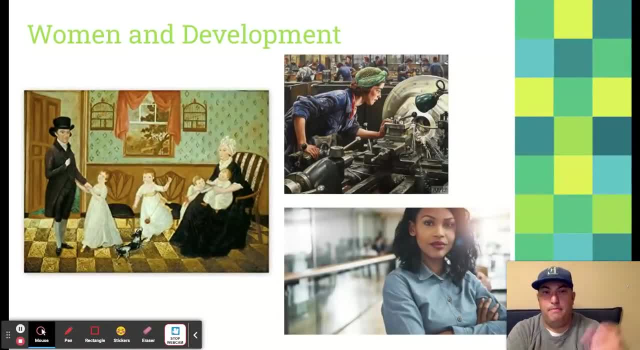 changing so that we can, we can allow women to be more economically successful, to tap into that economic potential and really like that, like life actualization potential. right, We don't want them just in the house anymore, We want them to live just as rich. 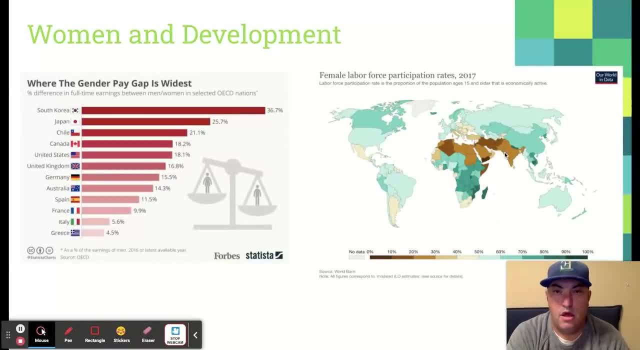 and diverse of a life as men do, right, All right. Now, one of the things that stands in the way of this is the gender pay gap. right, We got this chart over here that shows us where the gender pay gap is the widest. And take a look. These are all pretty developed countries, right? 36.7%. 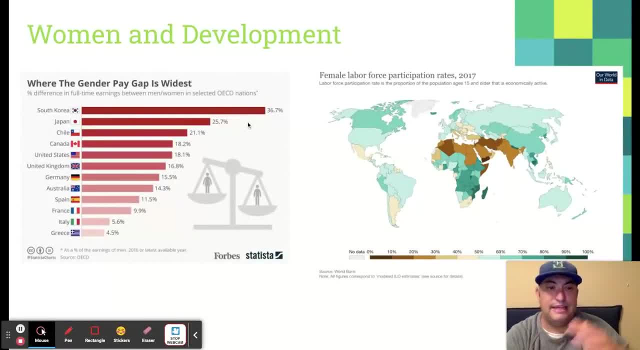 in that South Korea? Uh, measure right there, That's, that's huge, Right? So that again, if all people are little economic engines, then then that is really standing in the way of half of our economic engines, right, Um so? 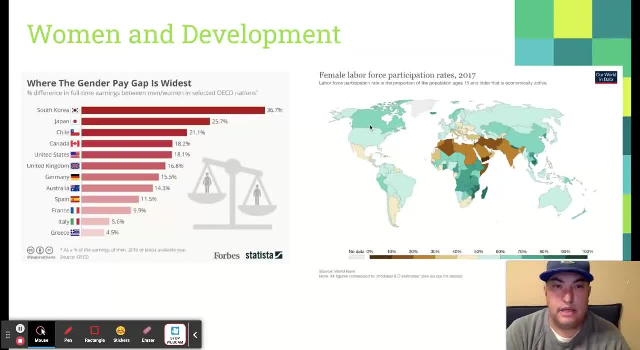 the gender pay gap is one obstacle. The other one is: is unemployment? Not in all, not in every place in the world do a lot of women actually participate in the labor force. All right, you see the brown, the brown colors down over here. 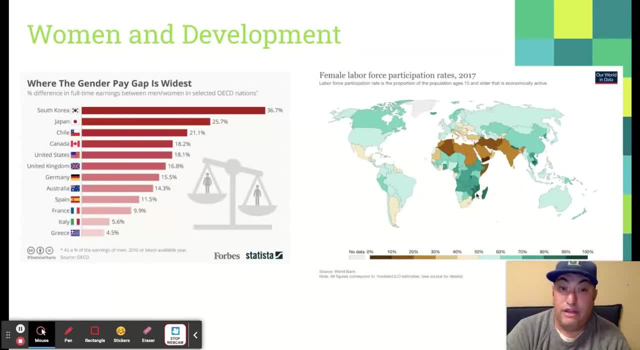 All right, so the gender pay gap is really standing in the way of half of our women actually participate in the labor force. All right, so let's look at this graph over here. Okay, I was actually kind of surprised by again this graph from for this map actually from our world and data. Okay, 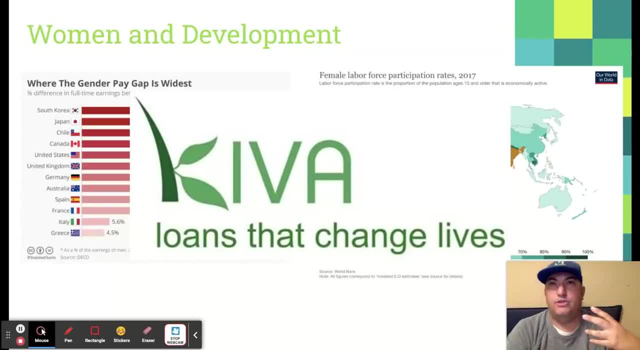 Now, one of the things that makes That like tries to kind of bridge the gaps here- See what I did. there are micro loans, and Kiva is an example of a firm that hands out micro loans to women, So that it's not like a big loan, but it's just something to get them on their feet, get them started. 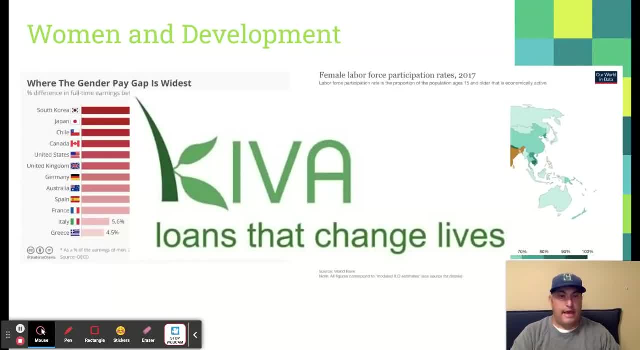 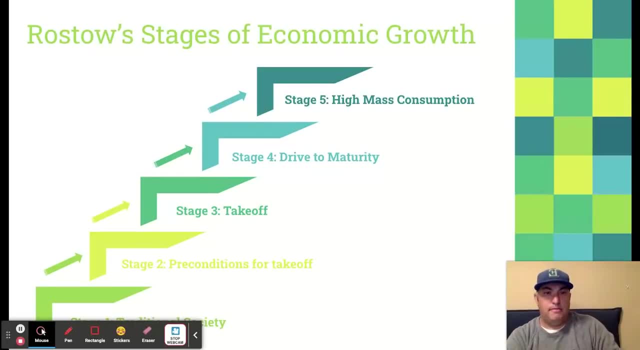 Maybe help them start their own business, Um, so that they can tap into that economic potential that we've been talking about. Okay, All right, halfway done, Let's get to some theorists. All right, Rostow. Rostow is one of the guys who got the shout-out in the CED. 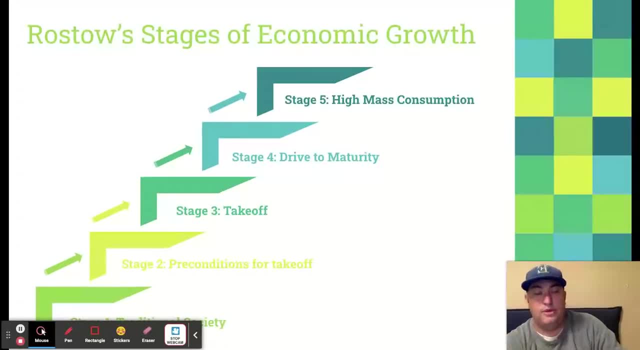 I don't know. Rostow, Did you do the Rostow Cup? I want to do that for the first time next year. You have a chance to do it this year. But you should know these stages of economic wealth right. Remember that, like economic, like that sectoral transition I was talking about, like this is: 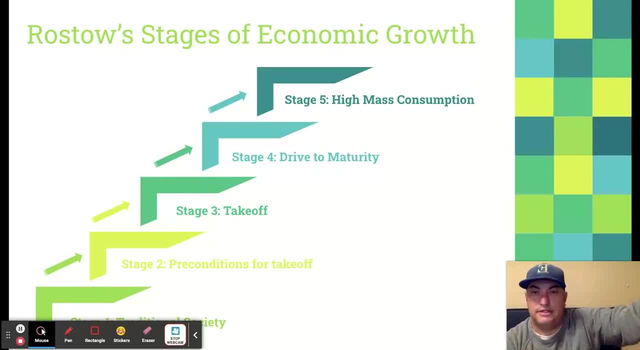 Rosso is essentially Done is. he's laid it all out for us in stages right. So imagine these countries at the very beginning of that economic sectoral transition. They're over here in stage one, stage two, stage three. They get to that takeoff stage. now They're industrializing. 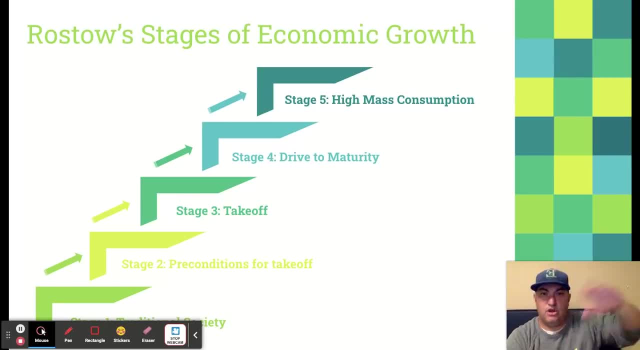 And then stage four and stage five is when they're making that switch over to that tertiary sector, And now they're really making some money. Okay, so Rostow stages of economic growth, make sure you know them. I don't think you need to really know the titles of them. 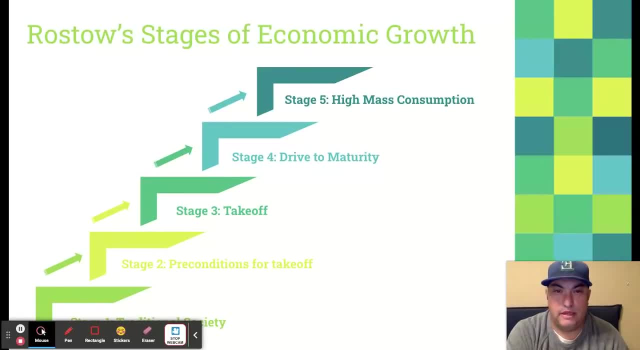 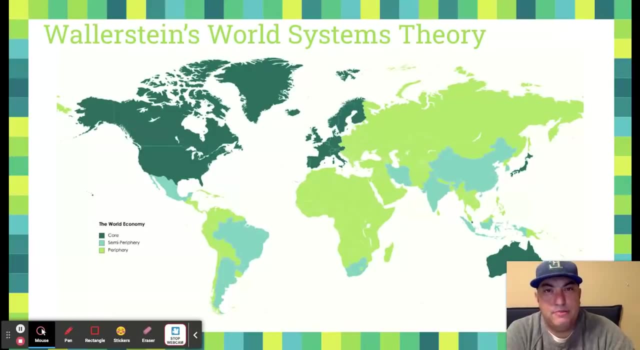 But you should know like kind of the difference between these, between these stages. All right, Waller Stein. Some of them are gonna say some of your teachers are placing Waller Steen. but I don't know, I was taught very little German as a young. 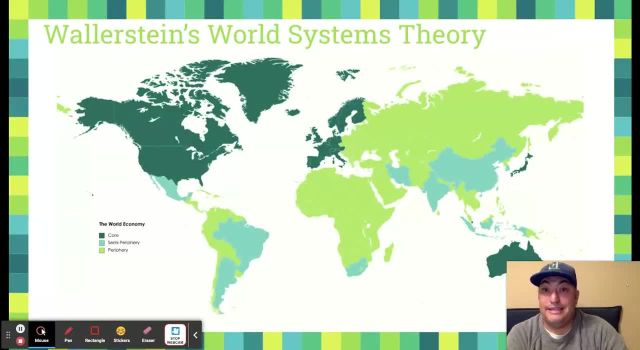 Californian dude, but I was always told my last name is fish. fine, like that. you take the The second vowel in that, in that a little chunk of the word, right there. So I think it's Waller Stein, Not Waller Steen, Waller Stein, but I don't know. I could be wrong. 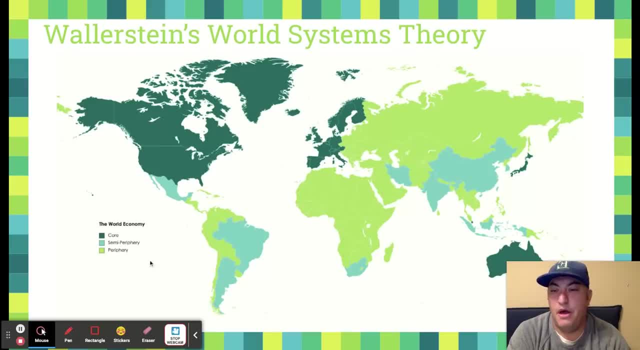 We'll have to ask him. I don't think we can, because I think he passed away a few years ago. but, um, What Wallerstein has is world systems theory. Okay, now, In the book that I like, in the textbook that I like for this course. 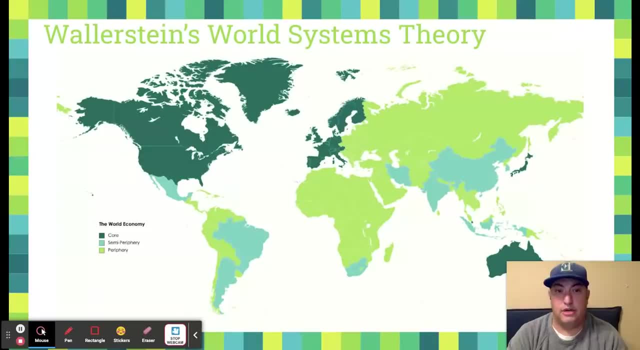 They put this in chapter one, because I think this is like fundamental to understanding the way the world works. so far right. Essentially, what Wallerstein tells us is that there is three groups of countries. right, We had the core right. we, these are rich countries. These are, these are the drivers of the global economy. 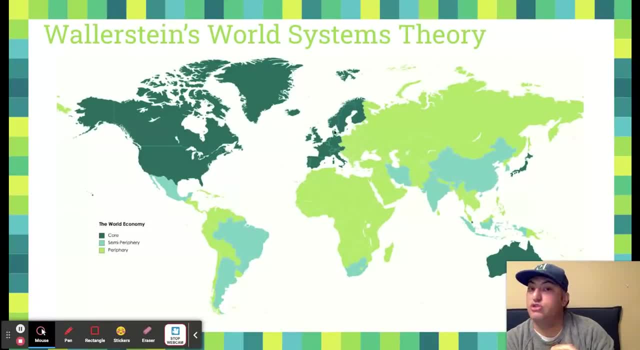 These are the big decision-makers a lot of the times. These are the countries that industrialized first. These are the countries that benefited the most from colonialism and imperialism. these are the countries that have essentially risen to the top of this global political pyramid by Exploiting other places. All right, and we call those places the core. United States will be a core country, Okay. on the other hand, 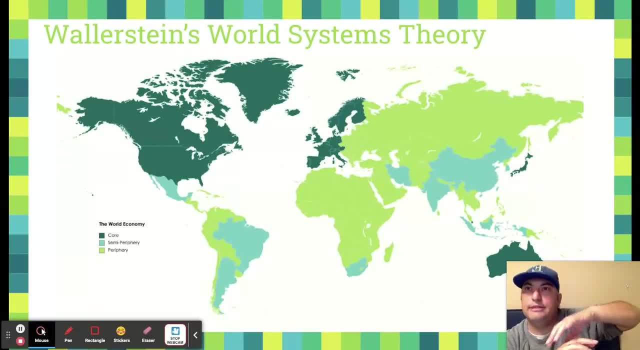 opposite end of the spectrum, We have those countries that were mainly exploited by the core right and that is called the periphery. Okay, so you see the vast majority of Africa's in the periphery, lots of South America, lots of Asia Beyond us, Russia, Lots of Southeast Asia in the Middle East. Those are those periphery countries. 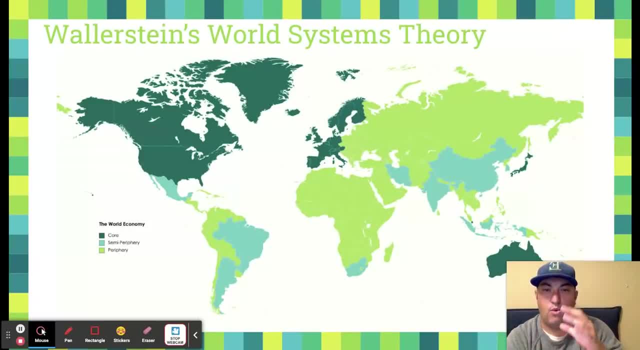 Okay, Now we have some countries that are kind of in the middle right. They're not quite core, but they're definitely not periphery. They're on the way to transitioning into some of those core countries, hopefully kind of lifting up the A lot of these people who live in these countries out of poverty, and those are gonna be semi periphery countries. 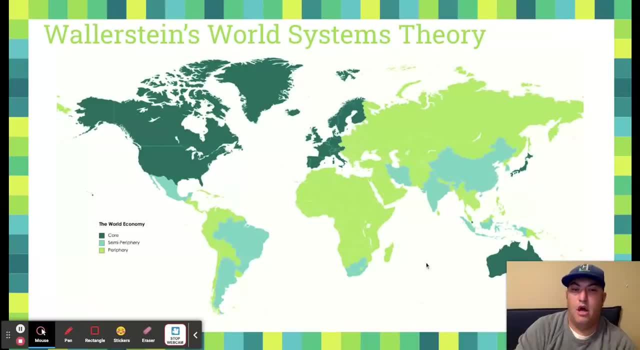 Okay, so like India, China, Mexico, Brazil, Argentina, Iran, Indonesia, South Africa, South Korea- I think that's all of them, but also don't get hung up like. I've seen a lot of different world systems theory maps as I prepare for this video, and 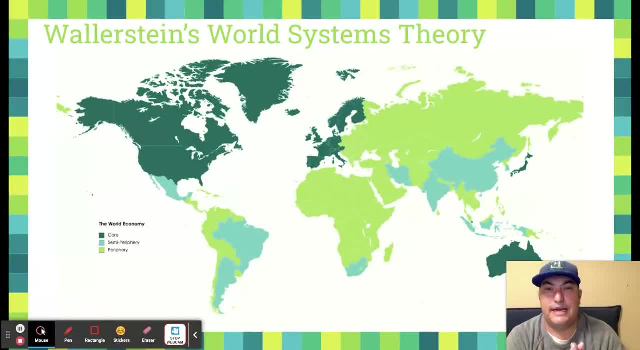 No one's gonna ask you what in what sector A specific country is in, because there's not gonna be a lot of agreement like a lot of like Eastern Europe. Sometimes you see this is core. sometimes you see South Africa as As periphery. don't get hung up on where individual countries are. I 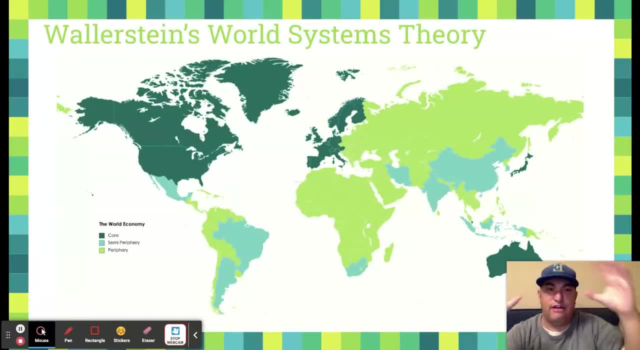 Would focus more on just like the, the theoretical, like groupings, Okay, like some are indisputable right, like the United States is definitely a core country, but some- you can go back and forth, But I don't think you need to get hung up on that. 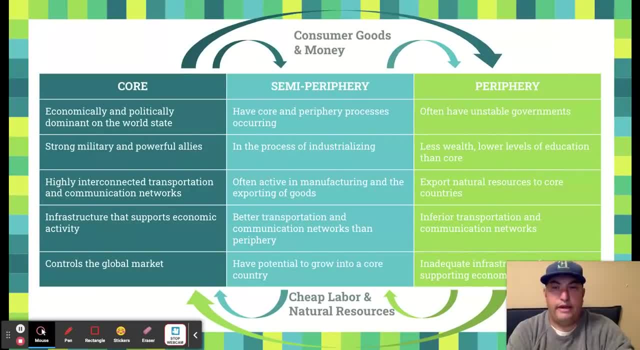 Alright, so this is another. I'm not gonna like go over every word here, Um, but this is another nice chart, Um, that I recreated for us, Um, That kind of goes into the difference between These three different groups- the core, the semi periphery and the periphery- and, most importantly, the main reason I wanted to put this in here. 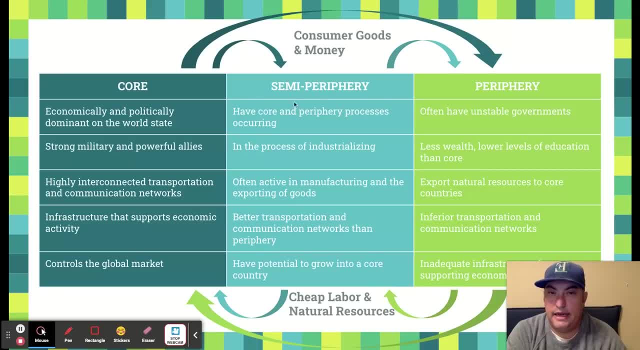 Is that? look at the arrows right. Don't get lost in the in the chart here, But look at what's going from place to place right from the core to the semi periphery, and the periphery are the consumer goods And the money, right you? you would think like: oh well, if the core is giving away money, like 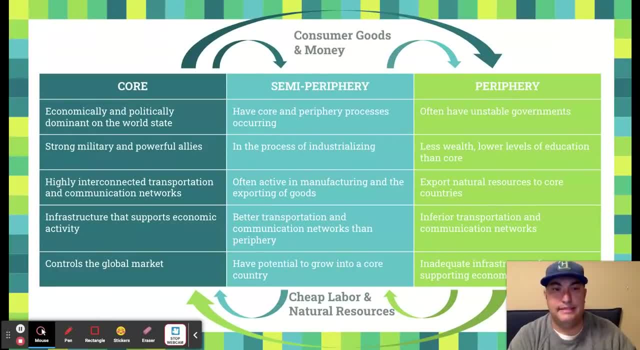 Doesn't. isn't that good for the periphery, the semi periphery? Yes, Yes, of course it is. but but the core is doing that to make their own right because they are getting back this cheap labor. they're getting back these natural resources at at such a discount here that they're able to 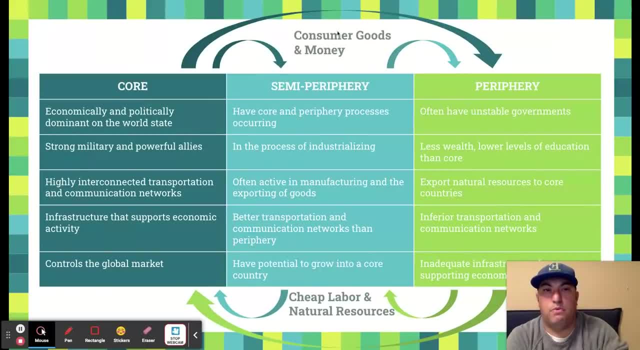 Just to sell these goods to those periphery and semi periphery countries and really take advantage of This situation. Okay, so feel free to pause the video right now if you want to take a longer look at the chart. I think that this is a pretty helpful one. 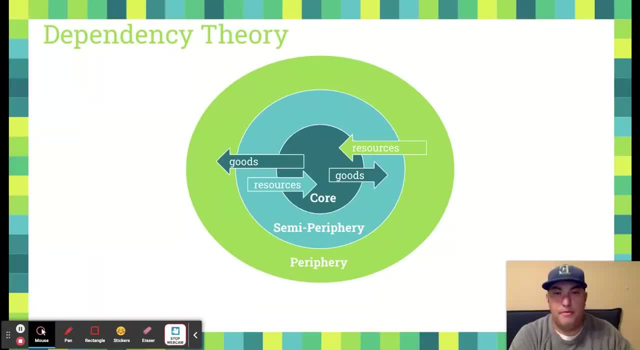 Okay, dependency theory. dependency theory kind of builds upon world systems theory on. We still have that core, semi periphery and periphery model right over there And it really is kind of showing how these periphery and semi periphery countries They get stuck right, they get dependent on. 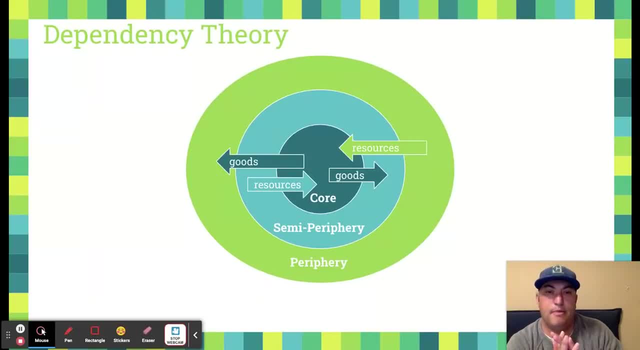 On the core right and they and to this less Or extent the semi periphery and it really makes it hard for these periphery countries to jump up to that next level. it makes it tough for the semi periphery countries to truly turn into a core country because you know they're 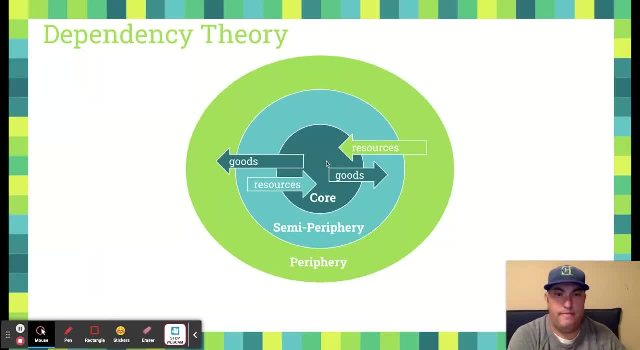 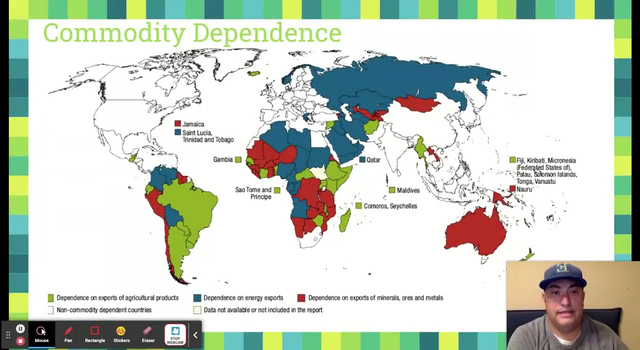 They're sending all their resources to the core right. So I think dependency theories is an interesting way of looking at things and and it really builds upon world systems theory from Waller or Stein Or Stein, I think- Fish. finally, I could tell you 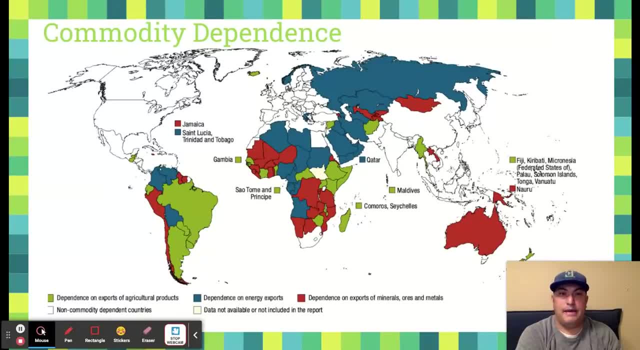 How my last name said it's fish, fine, All right. commodity dependence. We went over this in unit 5 right. when a country is is dependent on one commodity, It's like they're stuck only really like exporting coffee and like that's the majority of of how their economy functions. 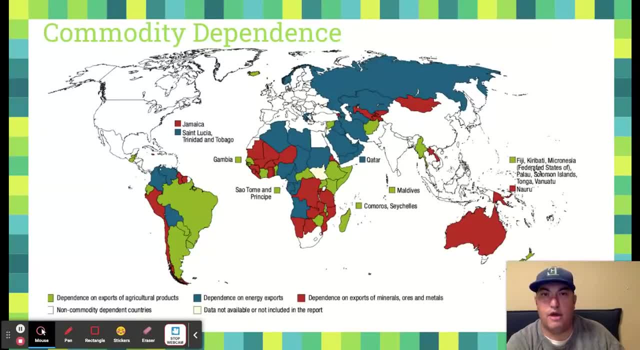 What happens if, because of climate change, we're not able to grow coffee in that region anymore? Okay, so these countries that are commodity dependent, Kind of like another, like a very tangible, effective dependency theory- Um, they're gonna be in a bad situation if, if climate change and other like maybe political factors change that they're not able to. 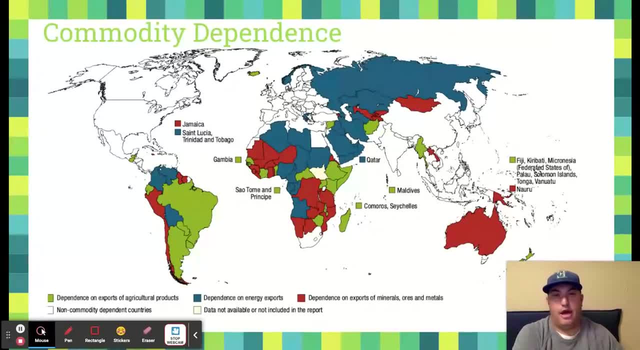 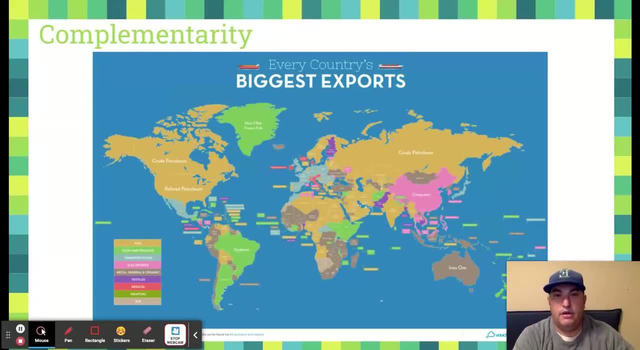 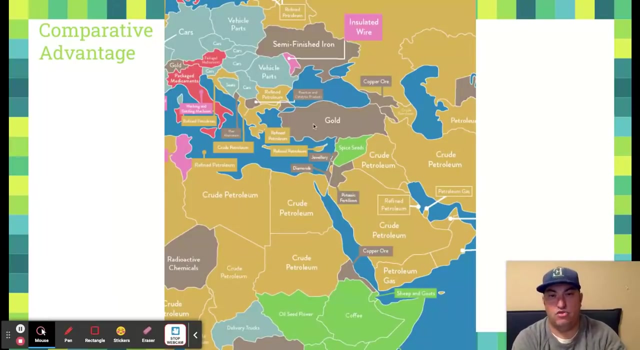 to really send out those exports That they're not able to. to really send out those exports? Okay, Complementarity. I found this map from The internet, of course. um, this is every country's biggest exports and zoom in. Alright, you know, zoom in on kind of like that Eastern Mediterranean region here, kind of like the triangle between 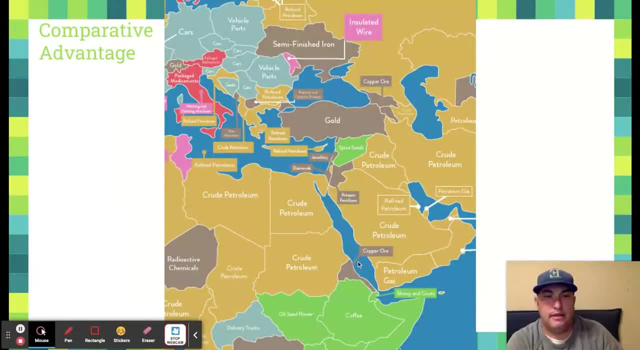 Europe, Asia and Africa here. and- and I'm just gonna like invent an example here, right for complementarity and comparative advantage on Ethiopia Makes a lot of coffee, great coffee made in Ethiopia and one of my favorite cold brews from one of my favorite coffee shops in San. 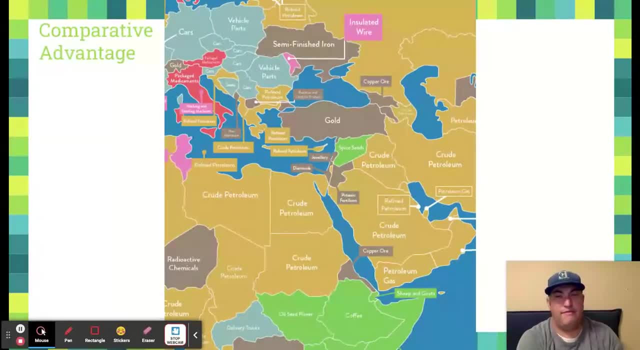 Diego that got replaced over once in a refill cafe. rest in peace. But my favorite cold brew from that place was called the Ethiopia right- great coffee in Ethiopia. What they don't make A lot of in Ethiopia, or at least according to this map, is cars. But they make it up there and in Germany right. So um. 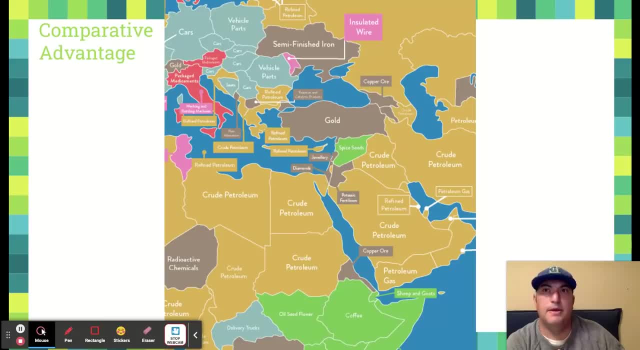 Ethiopia's got what we call comparative advantage, and in coffee, because up here in northern Europe It is gonna be way too cold, way too dry. It's not gonna be a place where a coffee plant is going to thrive. It's like actually literally impossible to grow coffee in Europe. right, Look it up. the coffee, though It's a thing. 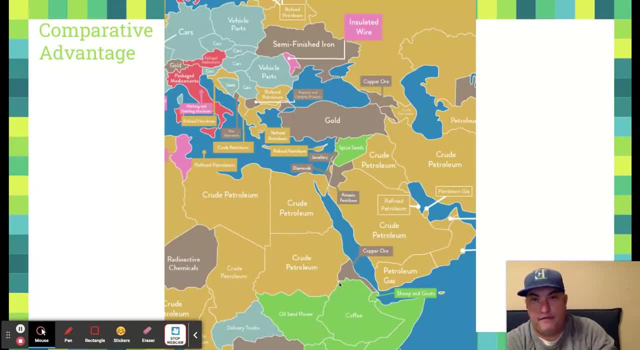 um. so Since Ethiopia has the coffee that the Germans want- and in Ethiopians They want to drive around right- They're gonna need to buy some cars. Maybe they want a Mercedes Benz. Germany's now got that comparative advantage in cars. one place wants what the other has, and vice versa. now We've got complementarity. 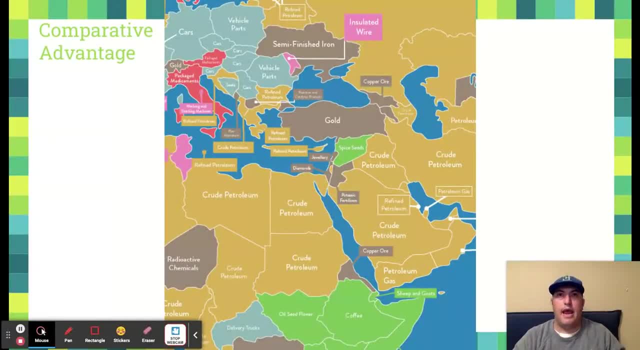 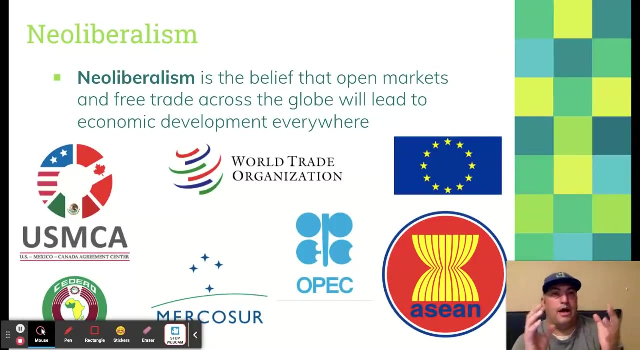 all right now we've got the Ability and the situation that is necessary for trade. Okay, So complementarity and comparative advantages like the, the bedrock of why people trade. I don't know those two okay. now when we get into, like, the global economy here and why people are trading and 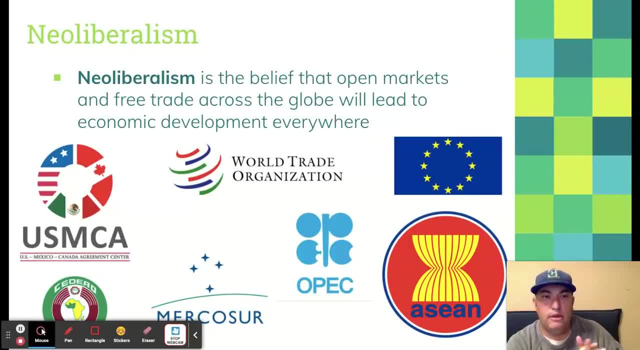 Breaking down barriers to those trades, we start to get into neoliberalism. Now I spell this one out for you, right? I spelled this one out for you because I didn't want you to get confused with, like the rule, conservative right, Like no. 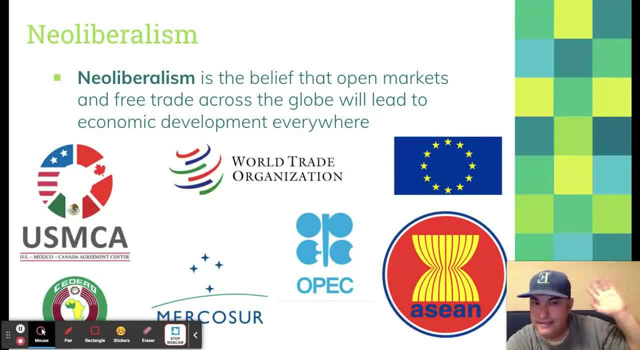 No politicians necessary here. We're not going to talk about that. That's, that's AP gov, That's hip Hughes. That's 12th grade at my school, right, This is not that all right, Neoliberalism. Neoliberalism is the belief that open markets and free trade across the globe will lead to economic development everywhere. 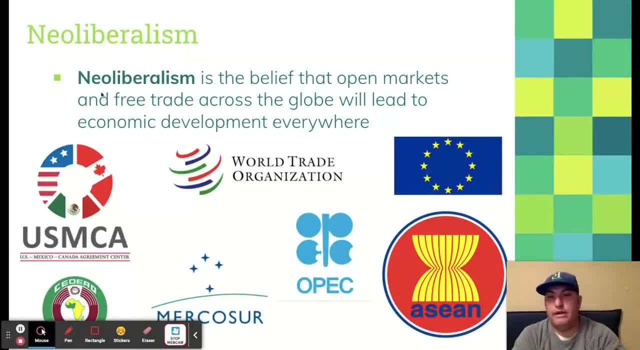 Okay. so you start to see these organizations, kind of like those super national organizations that we talked about in unit four, That they're really kind of band together To to promote this idea of neoliberalism, this to promote this idea that open markets and free trade are. 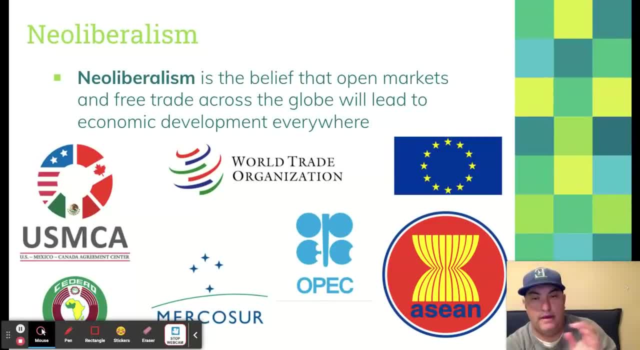 Going to be what leads to economic development. Okay, so there's a few in here that you should know. The World Trade Organization is probably the biggest and the most well-known. Most every country is nearly every country's, in the World Trade Organization. USMCA, that's like the updated version of NAFTA, like NAFTA 2.0 stands for the US, Mexico, Canada agreement. 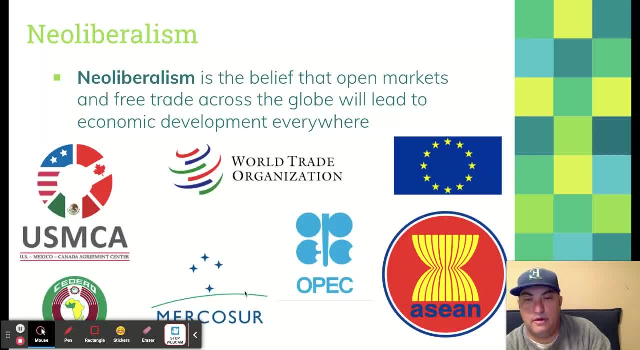 That goes over, stands for the Mercado Común del Sur of South America. We have eco was the economic coalition of West African states. European Union is one, a SCA n is one, And then the OPEC is a little on Unique, because it is focusing just on one commodity, one commodity only, just oil. 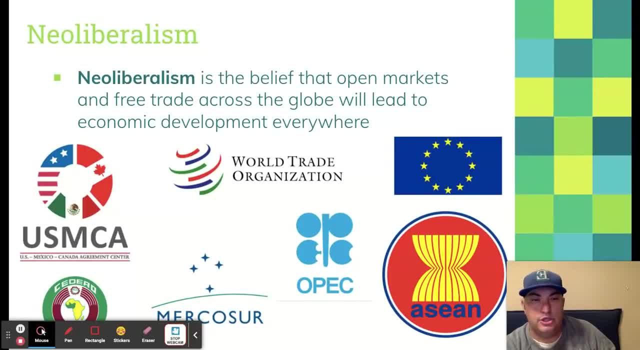 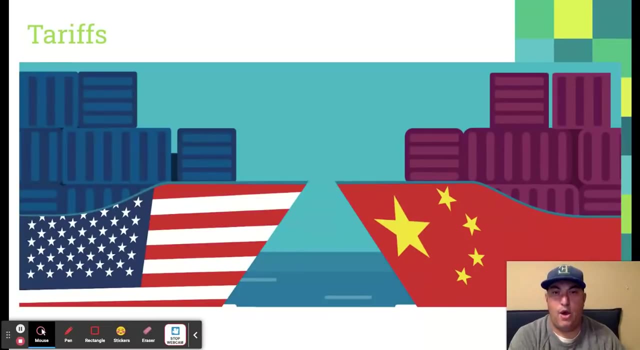 Okay, petroleum, all the other ones are going to kind of band together to to make trade for lots of commodities possible, But OPEC just concerns itself with with the oil. Okay, now, What a lot of those organizations do is work hard to try to break down. 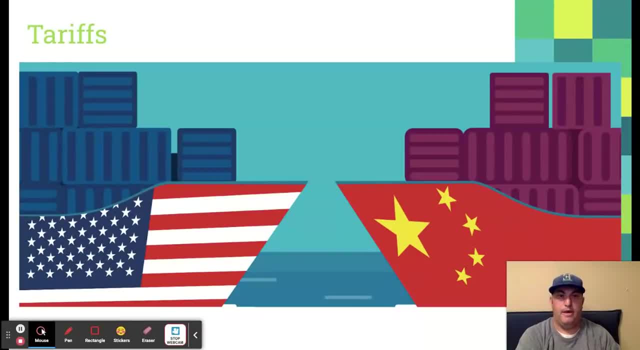 and convince governments to not have tariffs. okay, Very simply, a tariff is just a tax on an import right. So if we're the United States and we're getting stuff from China, Let's say, like for some reason we don't like China, Like maybe we're a previous president and like we're constantly feuding with China. right, 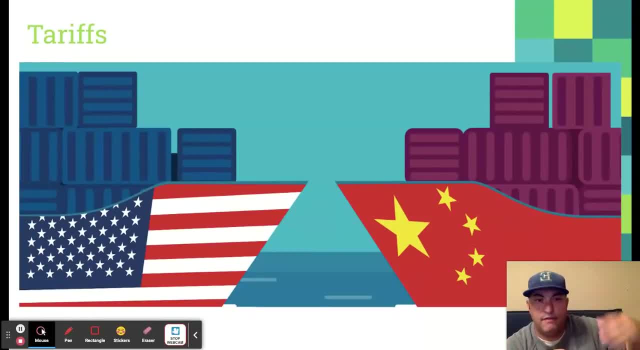 One of the things that the American government could do is slap a tariff on Chinese goods, And if you've ever looked at where your stuff comes from, you'll see that a lot of it comes from China right now. theoretically, This is gonna protect American producers, right? Why am I gonna go get my- I don't know my- t-shirts from China when I could just buy? 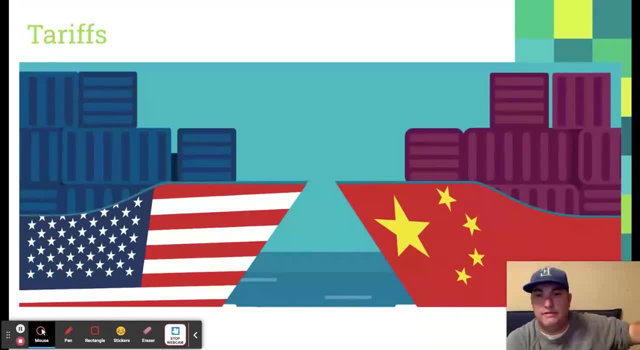 American t-shirts. right if that. if the Chinese t-shirts are too expensive, I'm gonna get them from. the American guys were selling it because their t-shirt I want to pay a tariff for. right now. What ends up happening sometimes- and this is what ended up happening in the most recent years- is that, well, China can make tariffs too. 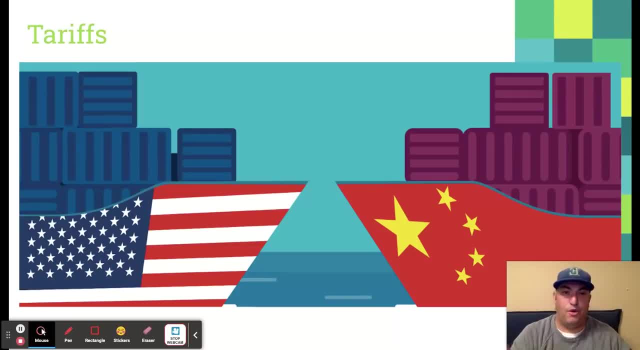 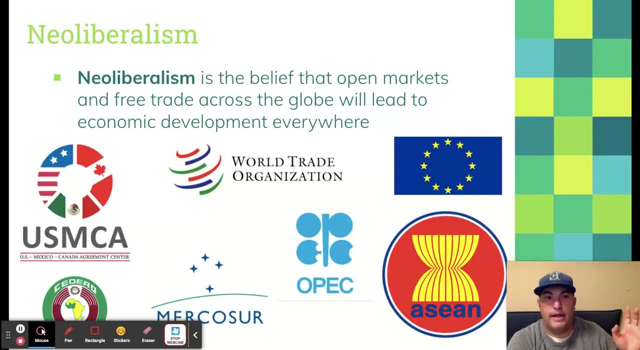 Right, China can put tariffs on American goods. So you start to get like this Exclude escalation here and if you and if you've heard of the term trade war in the last several years, That's what we get there. Okay, so these neoliberal organizations, they're not big fans of tariffs, right? 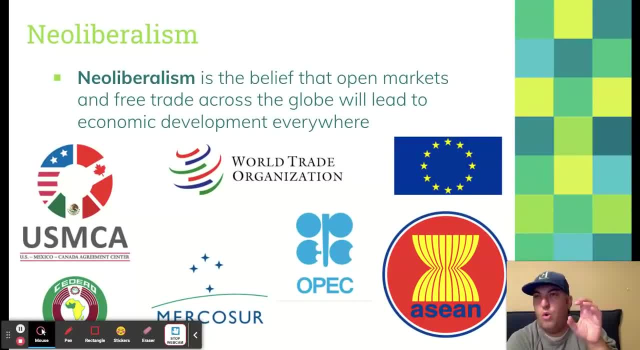 That is the government getting involved in trade. so they try to convince these governments to Lay off a little bit and not you create these tariffs, because that's not free trade anymore. right, That's the government doing in in putting its head with where the neoliberals don't think it belongs. 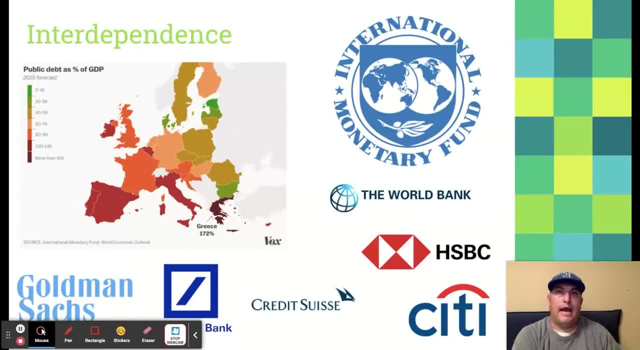 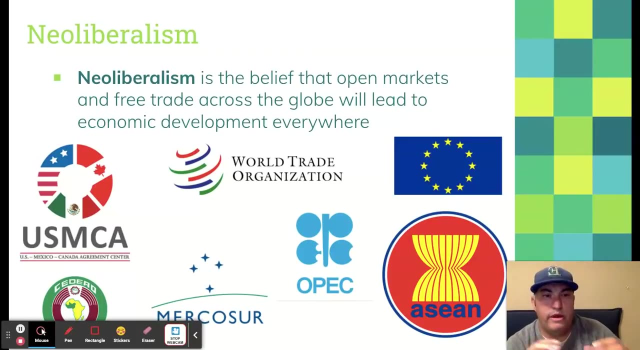 All right, so so, as you can see here, like the global economy is very interdependent, okay, we really depend on each other, especially when we're talking about tariffs, especially when we're talking about, like these are neoliberal trade organizations. we are making the economy, the global economy, so interdependent on each other. 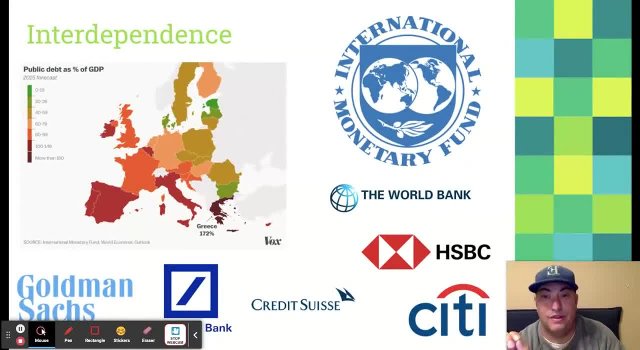 that if one domino falls or even, just like that, gets moved in the wrong spot, it can cause some some pretty harsh effects in the rest of the world. that's what you saw like with the Greek debt crisis. on you'll watch some videos. there's a cool one from from my, from my people over at box, about the Greek debt. 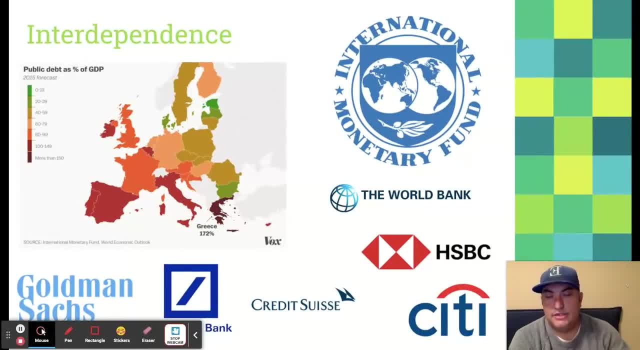 crisis on. but essentially, since Greece, like they're in the European Union, they're using the euro, but they don't have control over there. you're right, none of these states in Europe have control over the euro, so Greece needed to print its own money, essentially, but they didn't have that power. but it 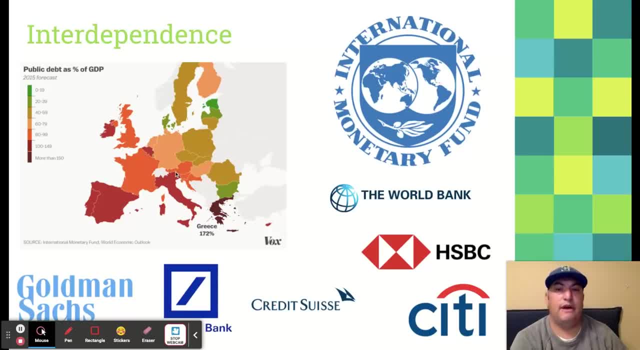 wouldn't made any sense for, like a journey or France, to print more money, devalue their currency, um they weren't in economic trouble. so, uh, greek debt crisis: look it up. that'll be a good example for you, for i don't know for q- if it comes up okay, and then you have um the imf. 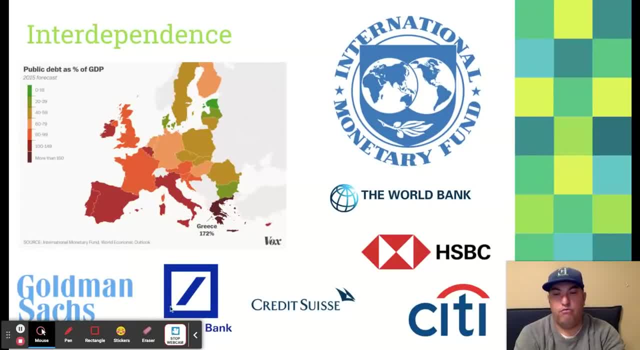 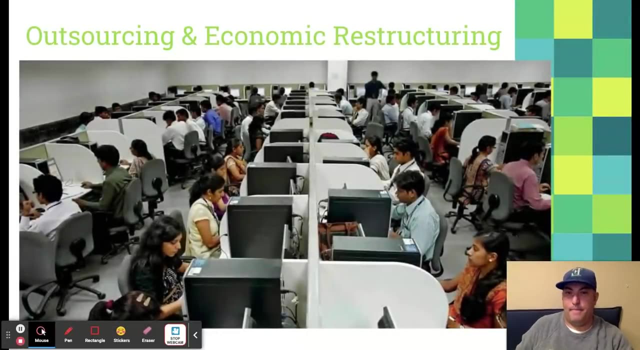 the international monetary fund and all these other like really high powered banks on both here in the united states and other countries that make lending possible, right that? and it really just is another example of interdependence amongst the world economy. okay, all right, let's more interdependence here, right, why? why are all of our jobs here in the united states going to other? 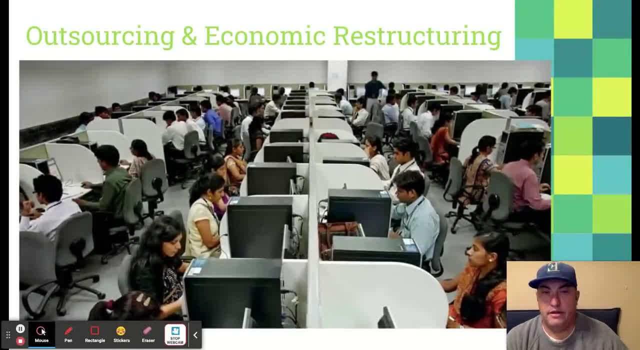 places, especially places like india, bangladesh, vietnam, china, it's because of outsourcing and economic restructuring. okay, so economic restructuring, like think about the structure of the economy, right, we used to have manufacturing jobs here in the united states. we used to have lots of labor and we used to have no labor. and i mean just remember we had the first one in 2019. 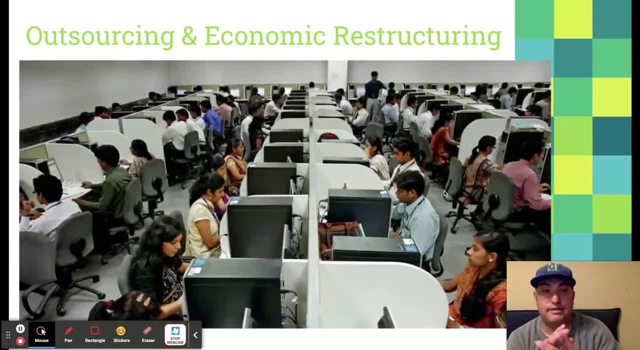 of like basic service sector jobs, like call sectors here in the united states. but these american companies have figured out. why am i going to hire an american for like 15, 16, 17 an hour when i could go hire a person overseas who already knows english and pay them maybe, i don't know. two: 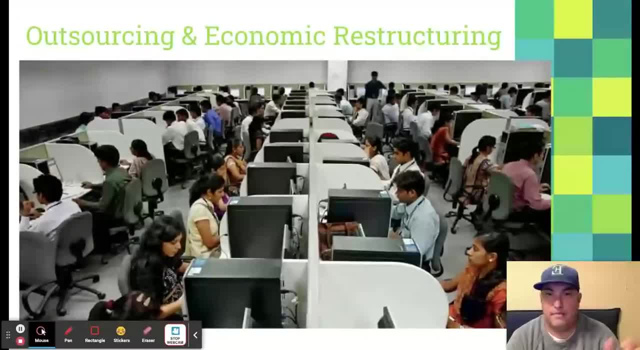 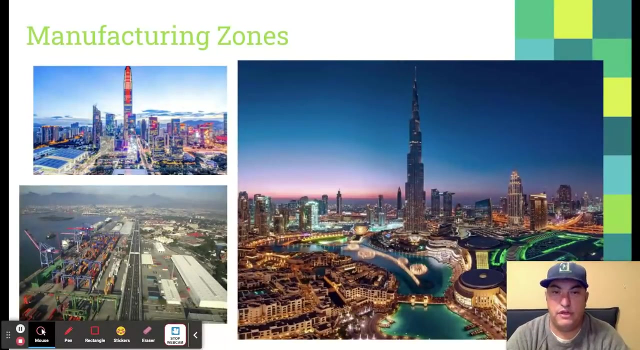 three dollars an hour, what's going to make more economic sense for them? okay, so you're seeing a lot of these jobs, especially in the manufacturing industry, especially like basic service sector jobs, going from more developed countries to less developed countries. okay, that is going to be economic restructuring. um, next we got manufacturing zones. okay, there's a few that you got to know. 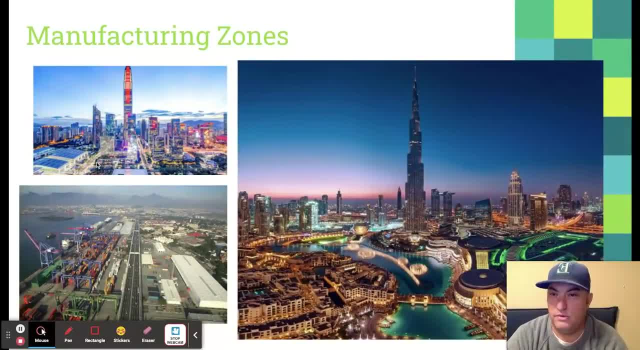 sorry i forgot to put the words on here, but we get special economic zones um, like in shenzhen, and special economic. special economic zone is a very like umbrella term. lots of stuff can happen in a special economic zone, but very basically it means that the rules of trade are different in that zone, in that part of that country, than in the rest of the. 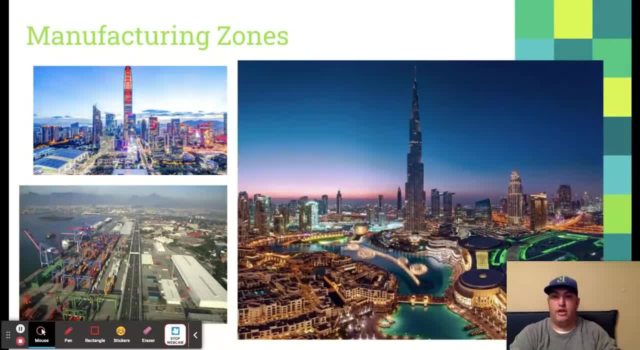 country right. china is very famous for using special economic zones. because they only want free trade essentially, in these special economic zones, they kind of want to, you know, make sure that they're controlling what's going on in the rest of china. but they want to make their money too, so 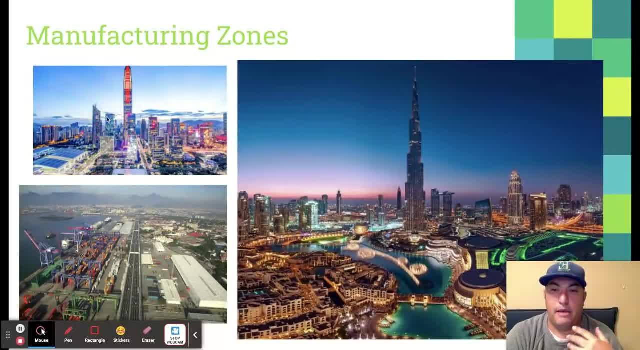 they create these special economic zones in places like shenzhen, where they're able to um to really have a real economy like that. uh, what else we got? we got um export processing zones like these down over here, um in rio de janeiro, um, and we also um have hold on, we're gonna have to pause here. 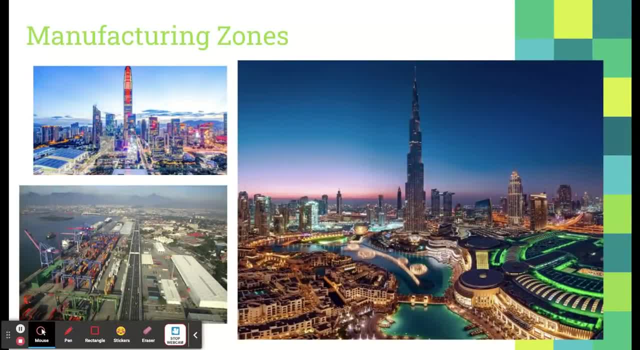 export processing zones. sorry, gotta look it up really fast, we'll get some water really really quick. free trade zones is the one that i skipped. free trade zones, all right, like in the united arab emirates, like in dubai, right here, um, basically they're really close to airports, really close to airports or other places where travel is going to happen. 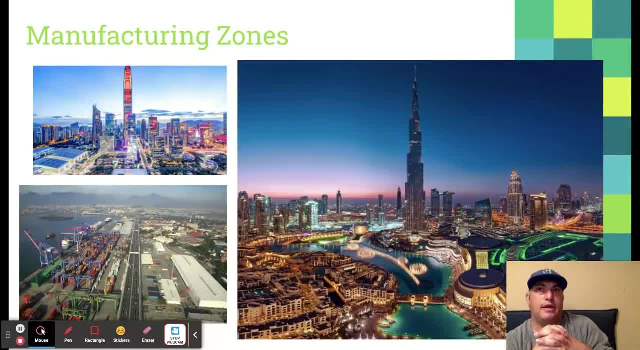 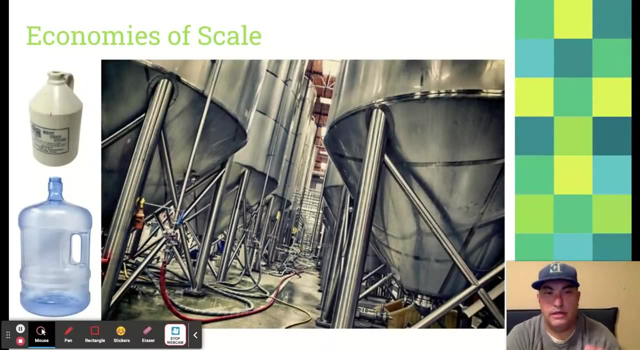 so that, so that travelers a lot of the time can can do their business, can get their, get their products without having to pay the taxes and tariffs, uh, that um are common in other places in the country. all right, economies of scale. so the next several slides are about things that are: 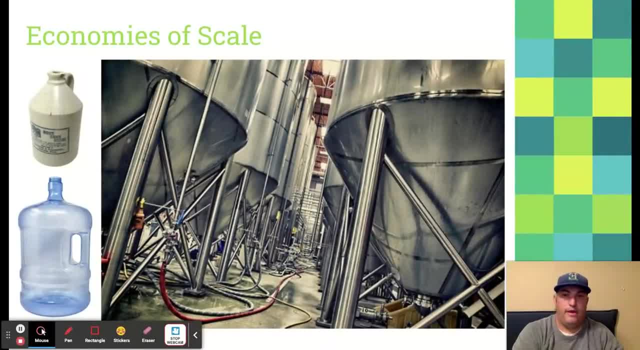 like gonna change our economic landscape here. okay, now my previous job, before i was a teacher. this is several years ago. at this point, i used to work at a restaurant. i wore a lot of different hats at this restaurant, but one of the things that i had to do on fridays in the morning is i would make the root. 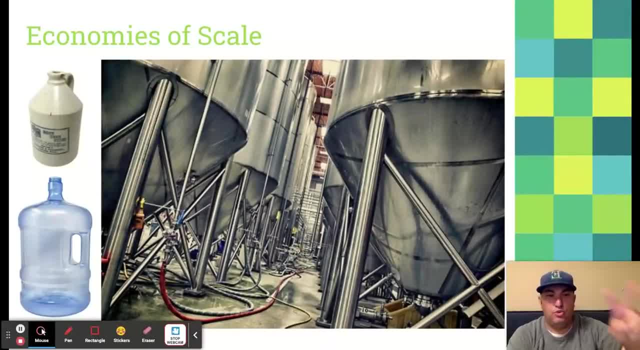 beer at this restaurant. okay, now, the root beer was only two ingredients here. right, it was root beer and water, and i would have to dump the little bit of syrup and a whole bunch of water and like one of these root beer tanks right here, and that took advantage of economy of scale. 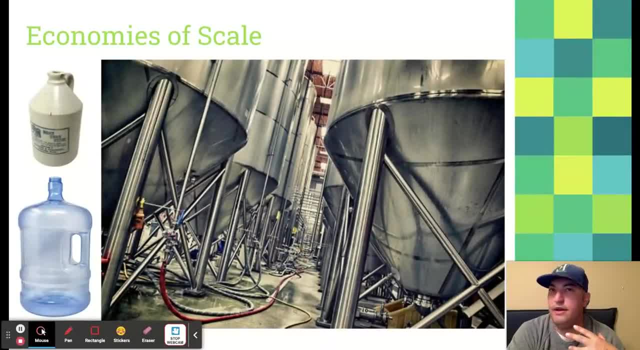 right because it made it so that the restaurant could, for a very cheap price, make a lot of root beer. right now you could just kind of like put the water in this here together in a cup and, you know, brew it together really fast and you got root beer right. but since we 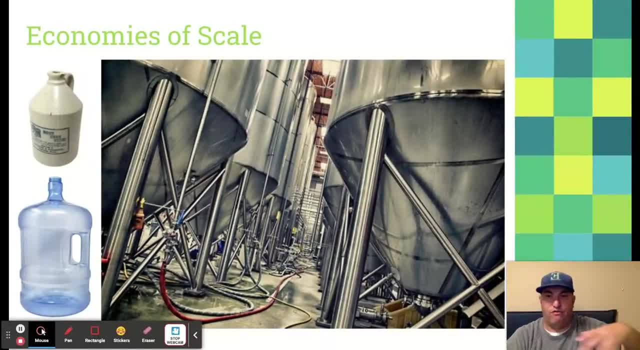 have the tank, the big, humongous tank that brews it together for us. well, we like to buy one of those. right, we like to buy one tank, and then we can add in all the syrup and all the water that we want and make as much root beer as we want. all right. so this idea that it's cheaper to make a second and a 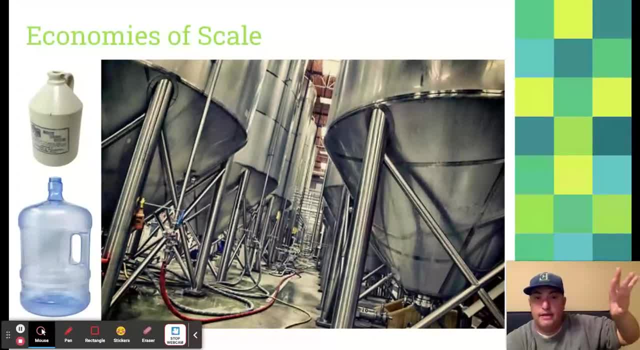 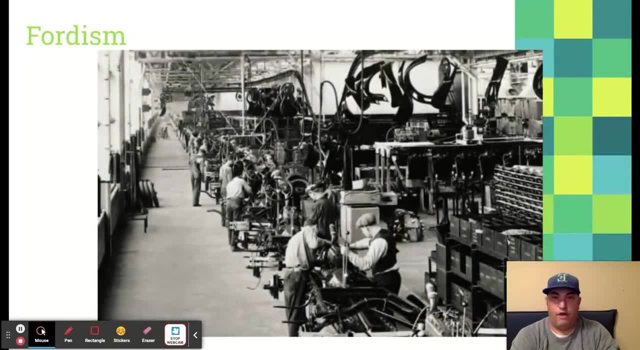 third and a fourth and so on, of a of a thing, of a commodity that is economy of scale. okay, and this basic idea leads to fordism, right, fordism named after henry ford. this is very traditional industrial jobs, right, everybody's doing one thing lots of times. you have this assembly line structure. okay, that would be. 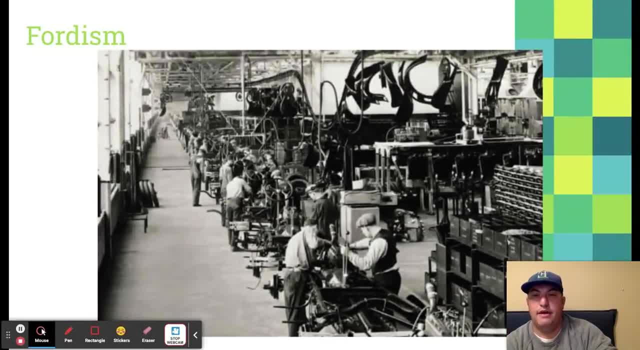 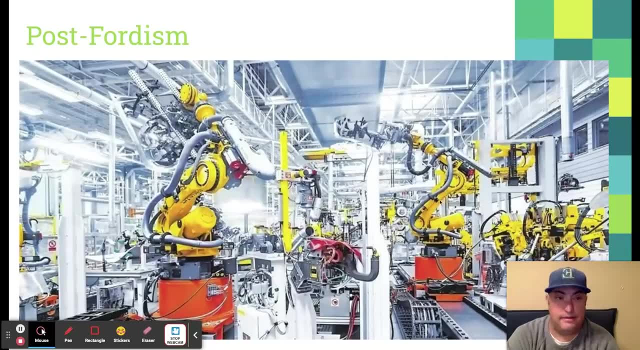 fordism, but we don't really do things like this anymore. right, because now we have a much more advanced technology and we're able to take advantage of post-fordism. right, it's not dudes and- and you know- actual people making our cars anymore. a lot of it is done by these very 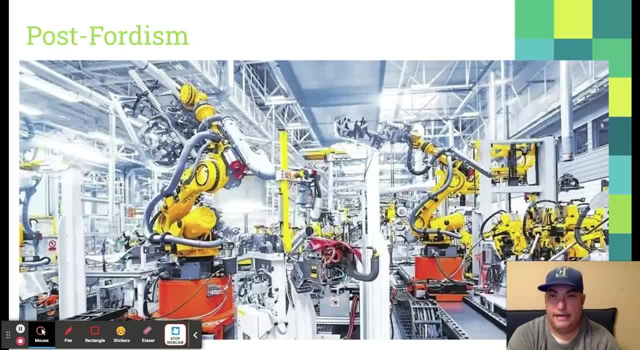 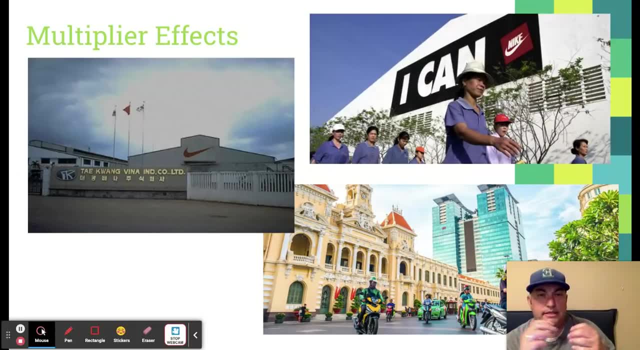 intense looking machines that i couldn't even like begin to tell you about. all right, multiplier effects is the next topic we've got to get to. okay, multiplier effects is. it's a pretty positive idea here. let's take a firm like nike. do you like nike? i love nike lots. 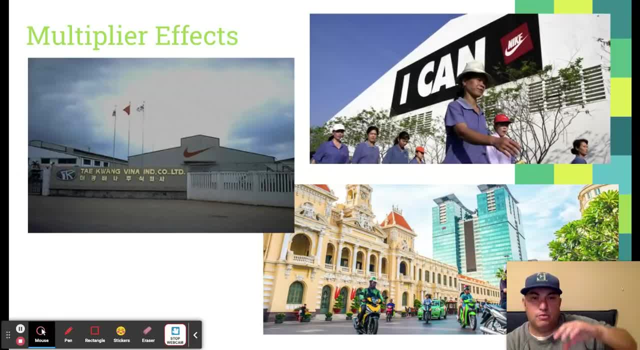 of nike stuff in my closet when nike goes abroad, when they leave the united states and and open up a factory in a place like vietnam, like what you see here. um, the idea is that they're investing into. ho chi minh city is where this factory is. their investment is going to get multiplied in. 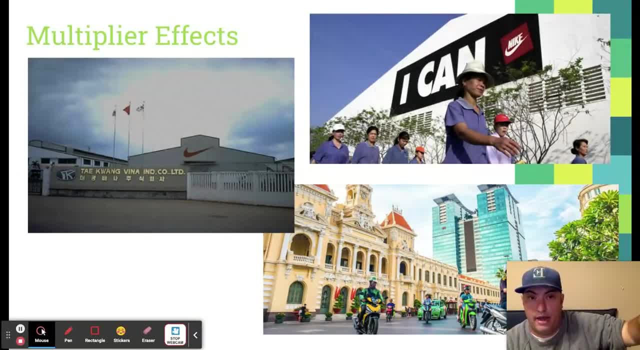 the local economy several times over. ideally okay, because not only are they hiring these people in another country, but now these people who are getting hired, they have disposable income, they want to spend that. they have to go to lunch, they want to go buy a house, they want. 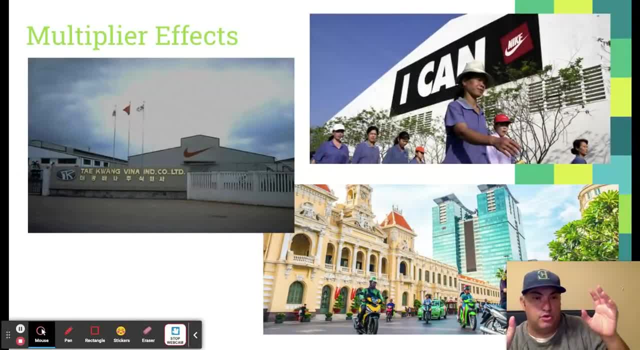 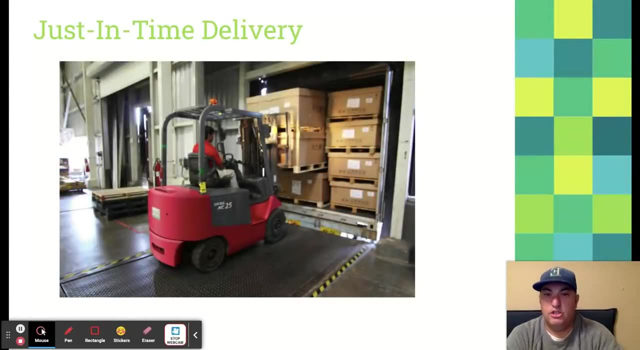 to go send their kids to college and, and that's going to create opportunities for um, for local restaurants, that's going to create opportunities for local businesses in that area and now they can invest more. that is all called the multiplier effect. all right, just in time, delivery. i gotta be honest, i don't know where this fits in. very well, this. 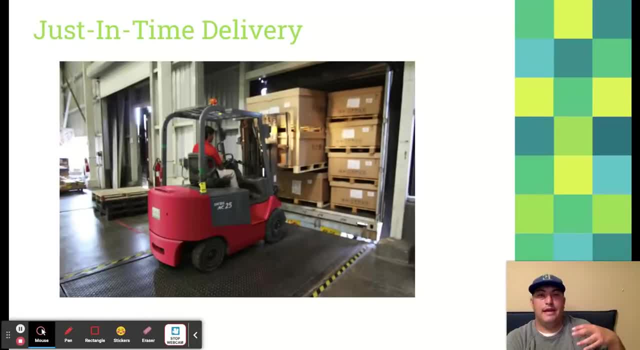 just kind of seems like a random thing to me. but just in time delivery: it's when these firms get the pieces to whatever they're making, like just in time, right, like right before they're going to make it, so they don't have to invest a lot in keeping a large inventory of of the 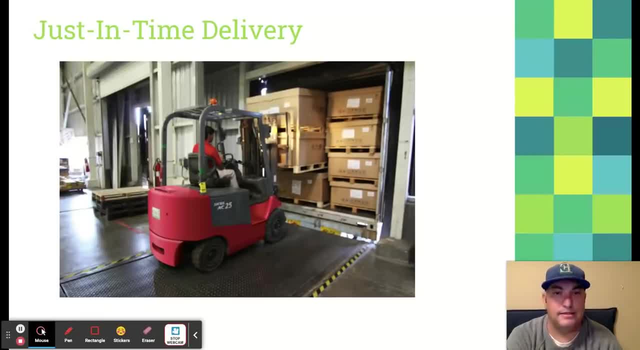 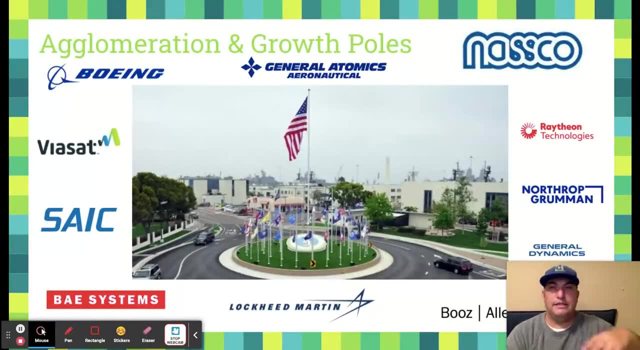 usual pieces or whatever they're making just in time delivery. i guess it's something geographers care about. okay, this seems more geographic to me: agglomeration and growth polls. okay, so this is like how, really like smaller cities, um like, try to get on the path to economic development. 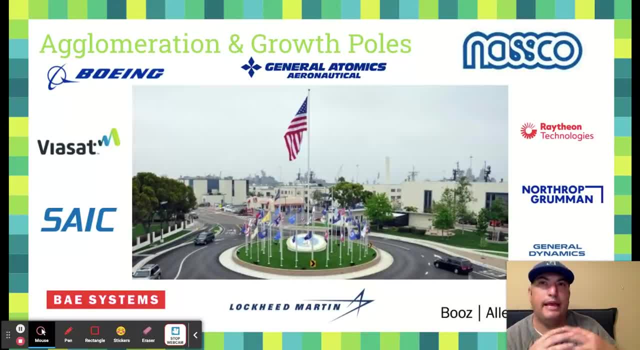 um, and what a growth poll is. it's like any like industry that kind of is like. it's like a main, like kind of like tent pole is how i understand it for the local area right in san diego where i'm from. our number one industry is defense in the military. okay, 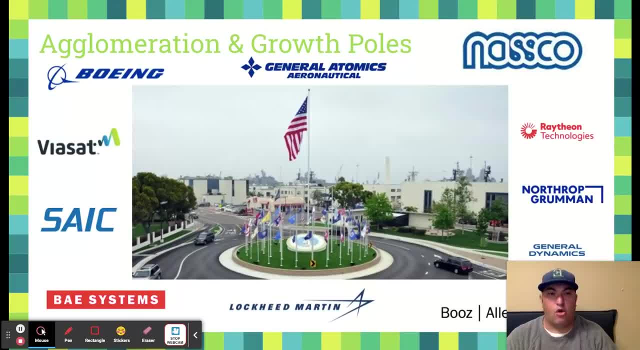 for obvious reasons. right, we have the beautiful san diego bay, great strategic location for a navy, for the american navy in our case, right now, because the navy has moved in and made san diego its home as a and you know other branches of the military as well. um, there's lots of firms here in. 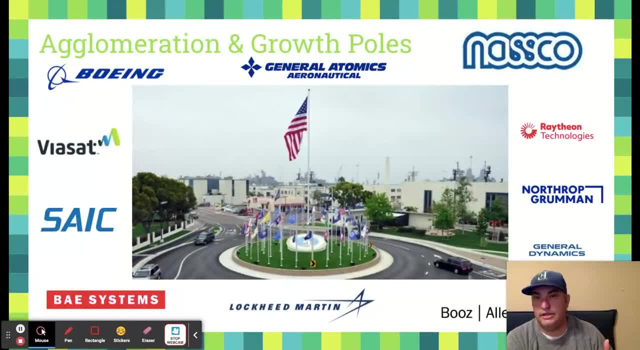 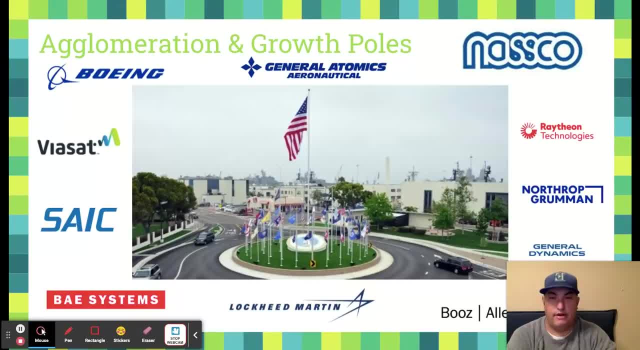 right, and you see the logos for a bunch of those um on this slide right over here. so they're either making ships like nasco or they're making weapon systems or they're doing some sort of engineering um, but it's a very. this is why it's such a big um. 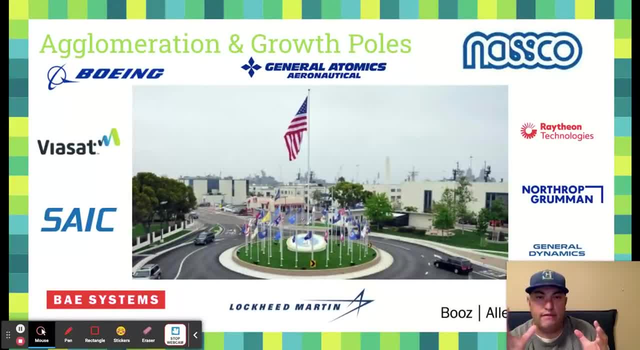 industry here locally in san diego, because they're all taking advantage, not just in the military- it's not like they just work for the military and that's it- but there's all these firms that are coming in and creating offices and creating job opportunities and really sharing resources and 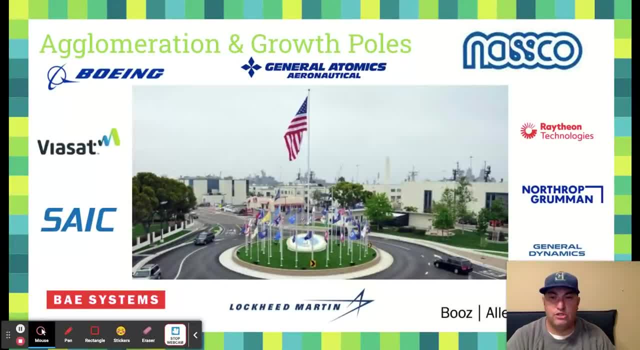 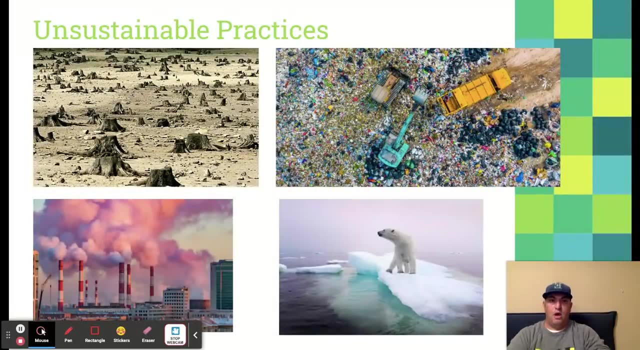 then that's where that word agglomeration comes in. they're sharing resources so that, um, san diego can be a very uh, efficient, uh, defense industry. all right, efficient spot for the defense industry. all right, just a couple more. here we go um unsustainable practices, this path to development. 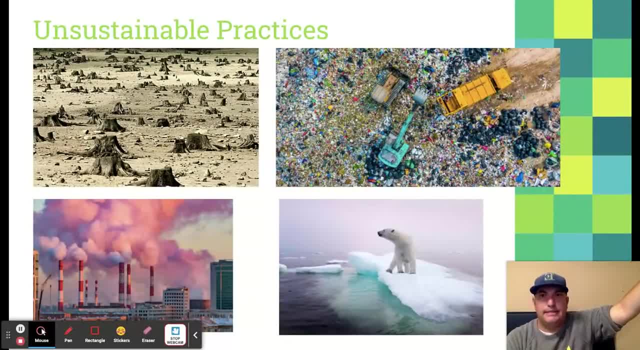 this path to industrialization, this path to development, this path to industrialization isn't great for the environment. right, resource depletion is what it leads to. pollution, uh, climate change, it's all like very unsustainable. so what our challenge is in the 21st century is trying. 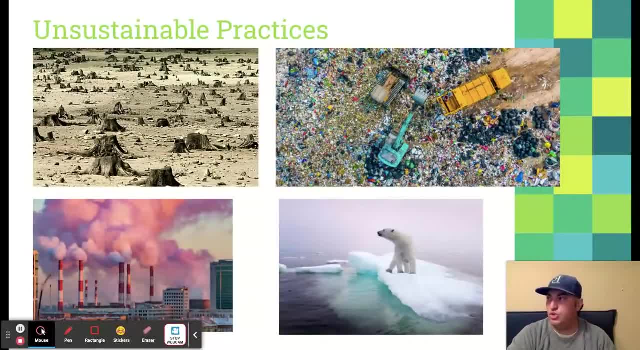 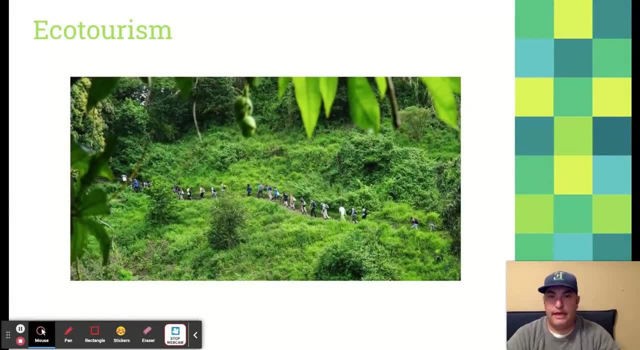 to figure out a way to do this development, to, to do industrialization, to make our money, without wrecking the environment at the exact same time. okay, ecotourism is is one way that's spelled out and that makes that possible, where people go to, to other places and they try to like be a tourist in. 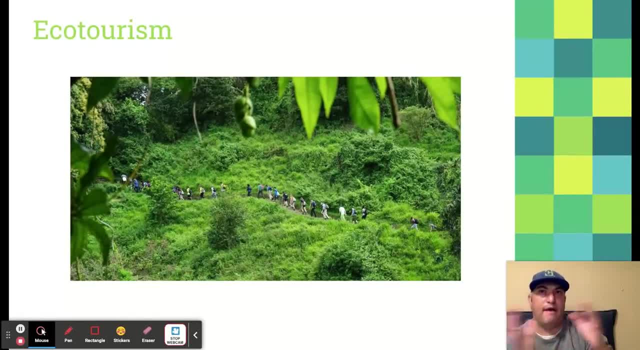 a more sustainable way. they're more in tune with nature, they pick up after themselves and really like they're injecting that money into the local economy. so the local, the local places can, um can be able to, to create an infrastructure to fight unsustainability on the road. okay, now. 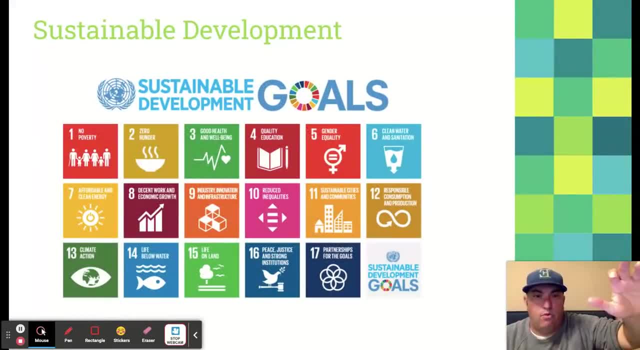 that. that's one small piece of the puzzle, though. here, right fortunately, we had the united nations um, and they created the sustainable development goals for the 21st century, and what's beautiful about the sustainable development goals, in my- in my opinion at least- is that you see all.